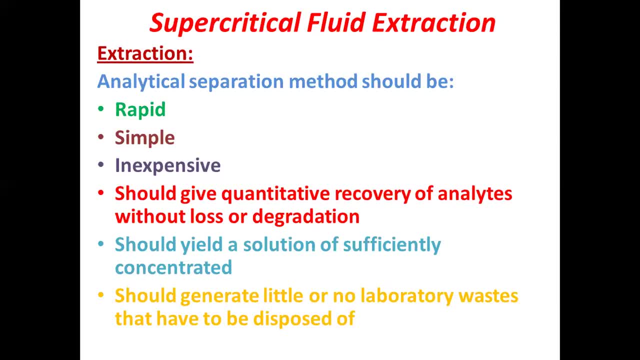 So, whatever the effluent obtained after the extraction process, at the end the extract must be sufficiently concentrated, Because if the concentration of the extract with respect to analyte is low, you will be going to increase the concentration. You may have to increase the concentration by concentration process. 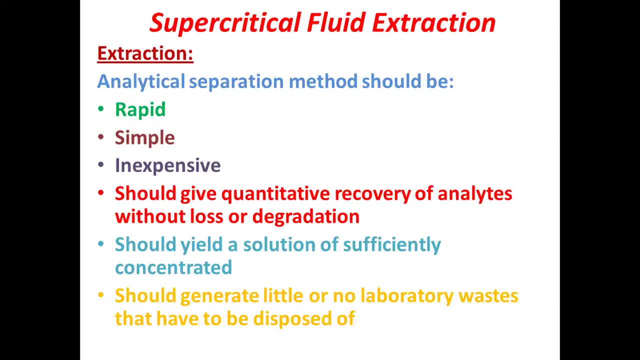 This is an added step and this is going to be highly disadvantageous, And after the extraction process is over, it should not generate any waste. If it is going to generate the waste, very little it should be. Therefore, the waste generated must be easily disposed to the atmosphere. 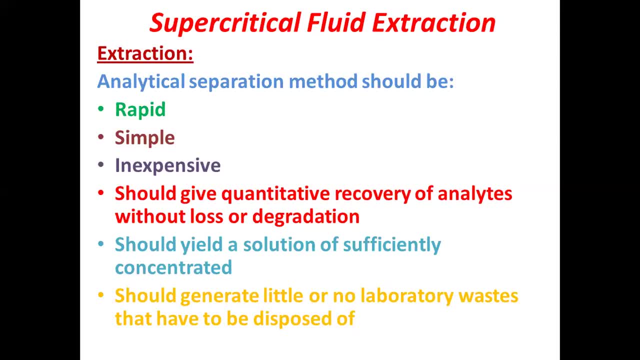 So you must expect no generation of the waste, or even it is generated to a very less amount. so any extraction technique you're going to adapt for the analytical separation, it should be rapid, simple, inexpensive. quantitative recovery of the analyte must be very easy, without the loss or degradation. 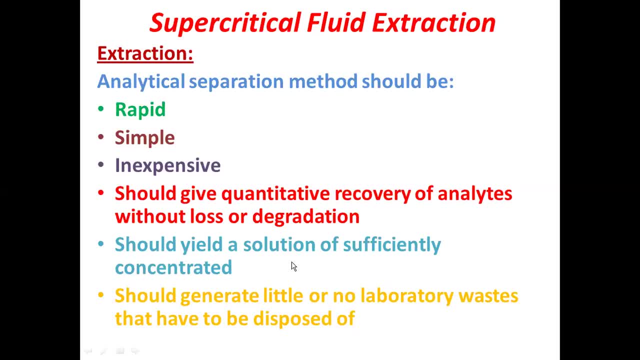 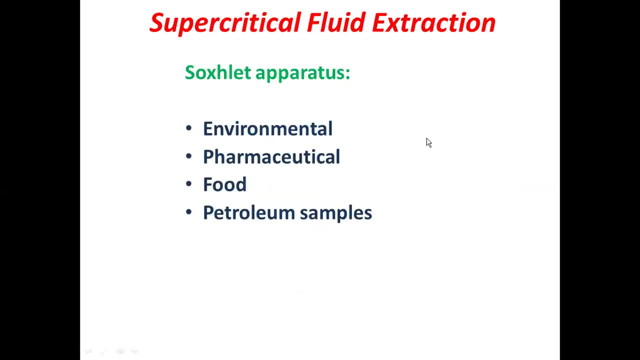 should yield a solution of sufficiently concentrated should generate little or no laboratory weights that have to be disposed of. you should remember. so the first extraction procedure started before all these, uh. ancient extraction procedures employed for the extraction process was saxlet operators. modern extraction procedures employed were liquid liquid extraction or chromatographic technique. 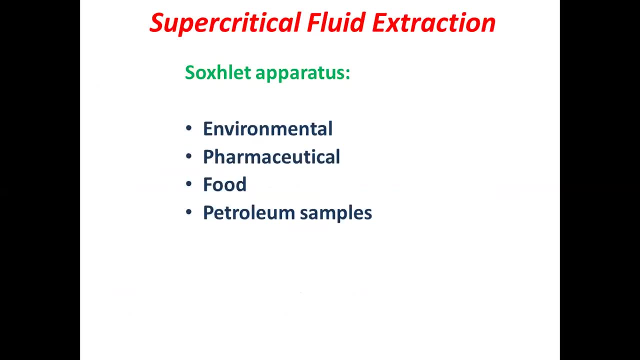 or solid phase extraction, etc. separation procedures will be employing liquid liquid extraction or solid phase extraction or supercritical fluid extraction, whatever it is. during the usual days when the separation science origin, saxlet extraction was one of the most prominent and commonly used extraction techniques for the extraction of environmental, pharmaceutical, food and petroleum. 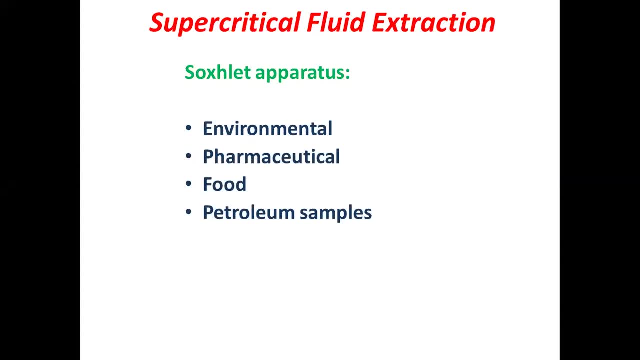 samples. whatever the sample origin. it may be from environmental origin or pharmaceutical origin or food, uh, a sample, it may be a petroleum sample, it may be. saxlet extraction procedure was able to be done. so you know the saxlet extraction process. uh, as your chemist, you might have seen the saxlet extraction. 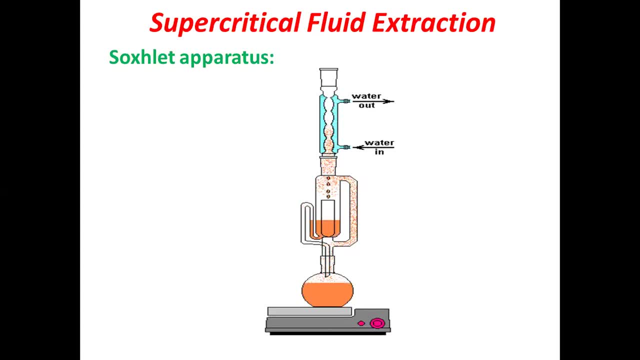 operators. you can see here an animated video showing how the extraction process is going to be done by means of saxlet extraction procedure. so it requires a reservoir- solvent reservoir- this is a condenser- water cool condenser- and this is a saxlet operators. the intermediate unit will be a saxlet. 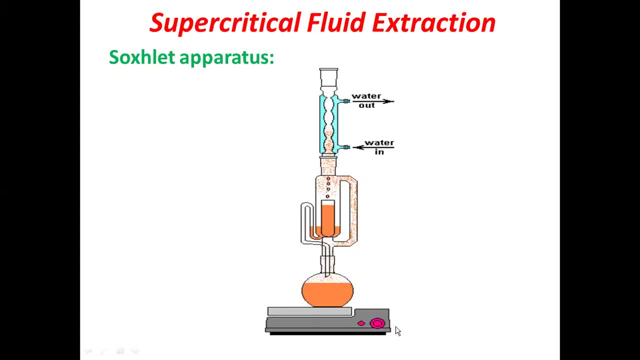 operators. so this is a hot plate. even heating mantle can also be used. this is the sample chamber in the saxlet operators. it is an intermediate unit of the whole operators in the saxlet operators. the sample is taken in the sample unit. sample is taken in the sample unit. from this sample we are going to extract: 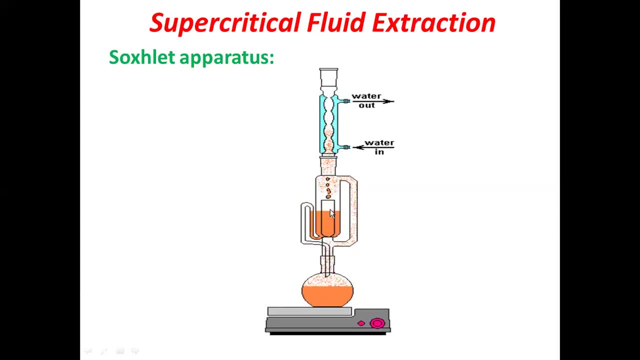 the analytes by saxlet extraction procedure. so what we do here? the sample unit is extracted in a box and then that sample is going to be taken in the solvent reservoir. we will fill the solvent. we will fill the solvent. a water cool condenser is fixed because we will be heating during the extraction process. 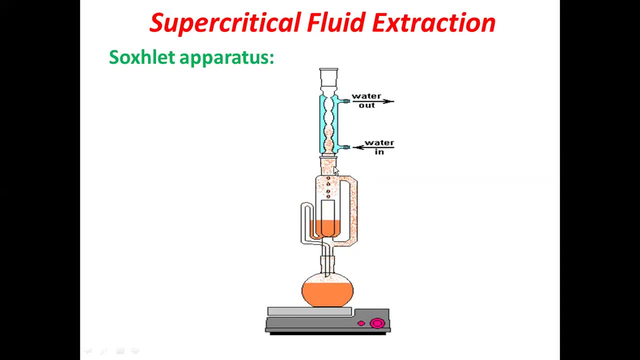 the solvent is going to be converted into vapors. after getting condensing vapors into liquid, that liquid is going to be interacted with the sample which is present here. so, in order to do the condensation process, the condenser- water cool condenser- will be used here, and this condensation 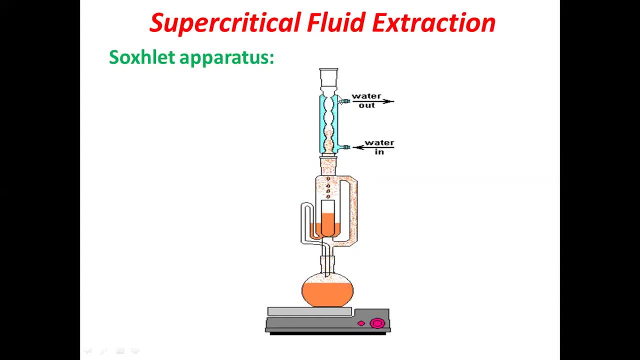 will be done by passing the water through this particular condenser. so you take the solvent reservoir, you take the solvent reservoir, you take the sample in the saclet operators, fit into the solvent reservoir and to the saclet operators you fit water cool condenser when you heat the solvent. when you heat the solvent, 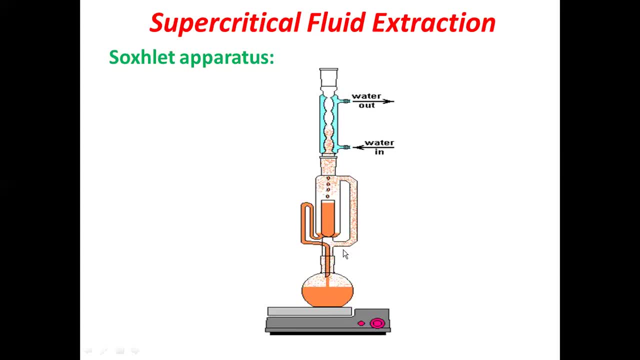 solvent is going to be converted into vapor. solvent is going to be converted into vapor and it will condense back to the sample unit here and the analytes, whichever having the selectivity to get dissolved in the solvent, they are dissolved in the solvent. therefore, liquid in the sample unit will be increased, will be increased and, as a result, as a result, 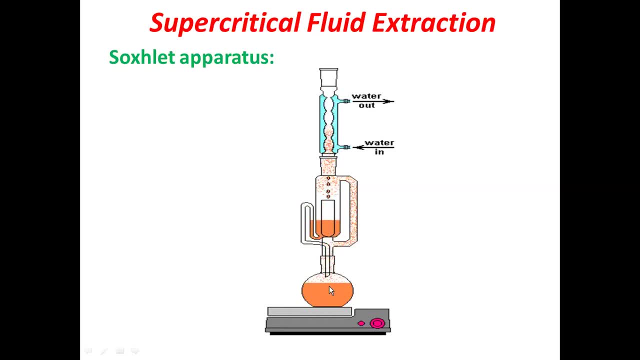 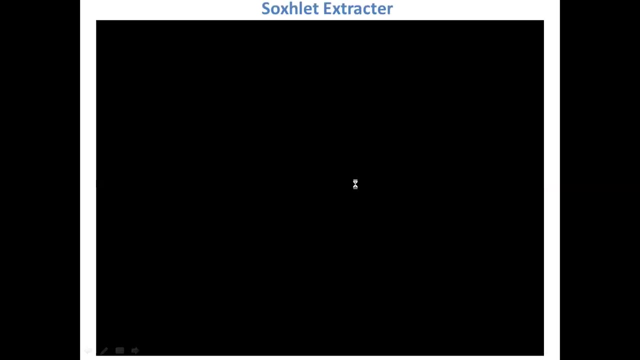 the solution is coming back to this solvent reservoir. so whatever the solutes separated will be collected in this solvent reservoir only. so this is the operation of the saclet extraction procedure. you can see here a stepwise assembling of the saclet operators and how we are going to utilize the saclet operators in order to perform the separation. 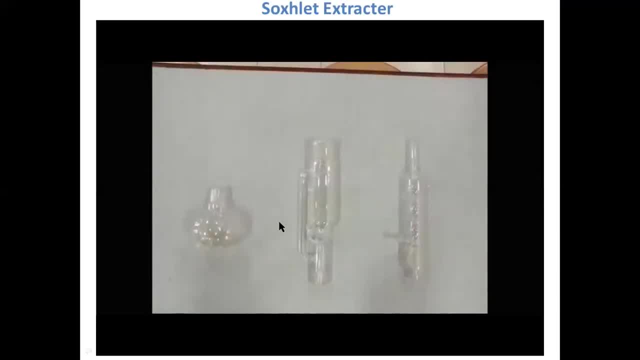 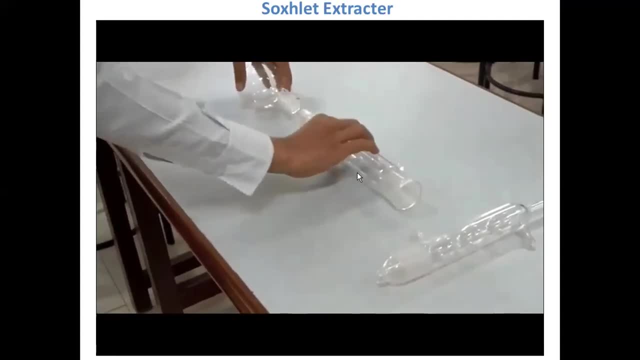 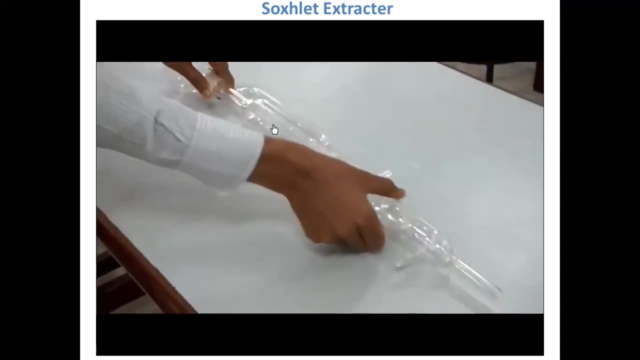 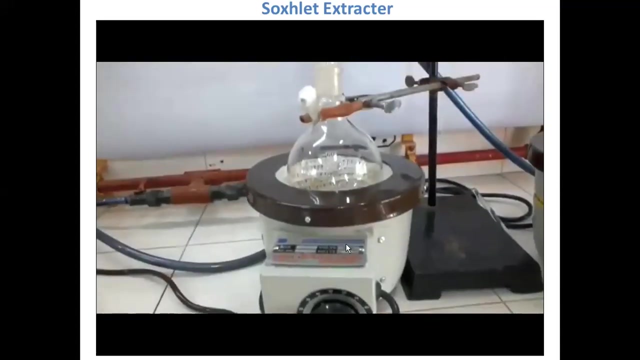 process. so three components are required in order to perform the stock slate operation. uh, one is the solvent reservoir saclet operators and the water cool condenser. so inside the satellite operators you can see a sample holder. you can see how these units, three units, are going to be assembled one by one. 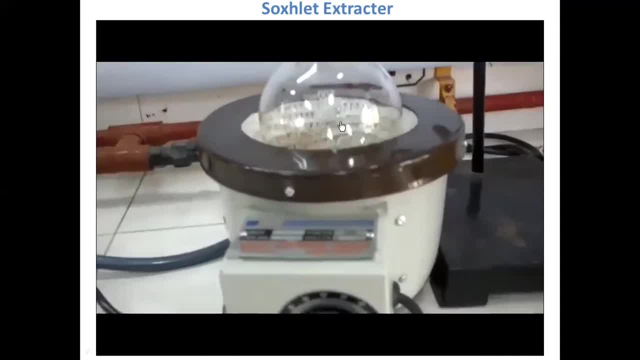 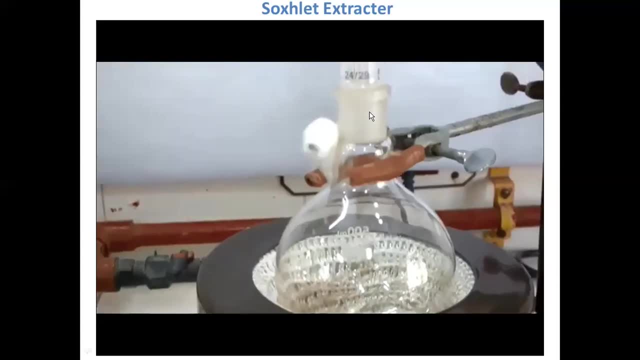 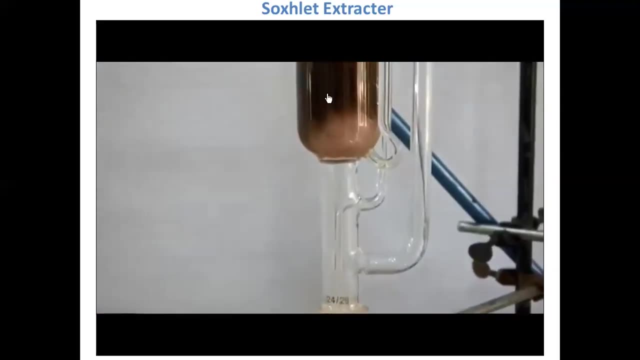 This is an heating mantle into which the sample solvent reservoir is going to be placed. It's containing the solvent, several milliliters of the solvent, Into this solvent reservoir. the soxhlet operator is going to be immobilized, So load the material in the sample compartment. 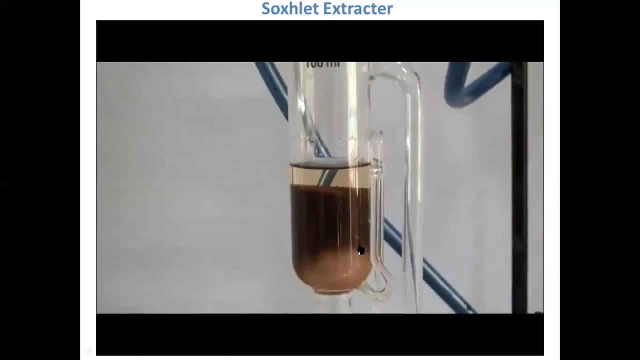 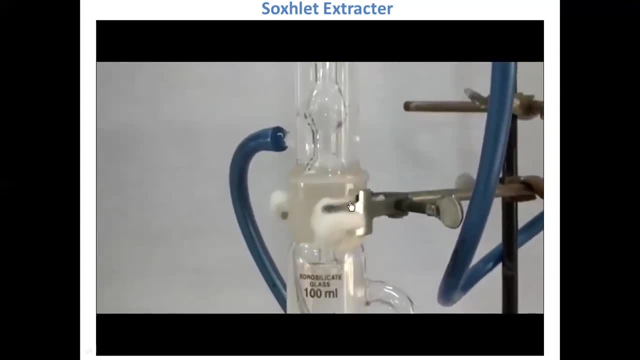 Prior to fixing the soxhlet unit to the solvent reservoir: you take the sample in the soxhlet operator, that is sample compartment, and fix the sample compartment by means of water-cooled condenser. This is going to be the water-cooled condenser. 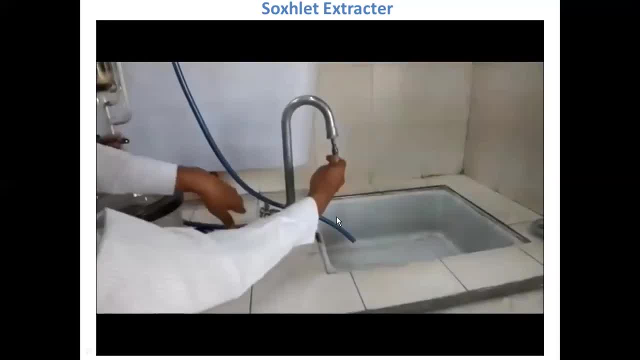 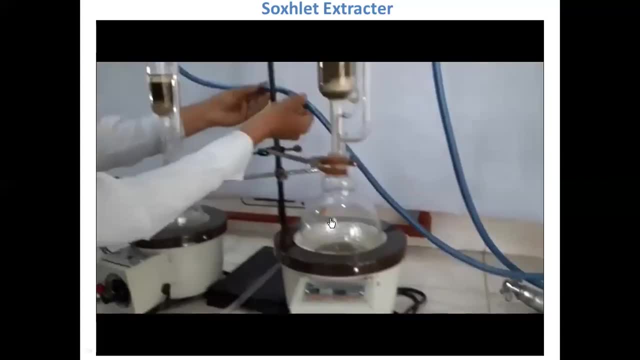 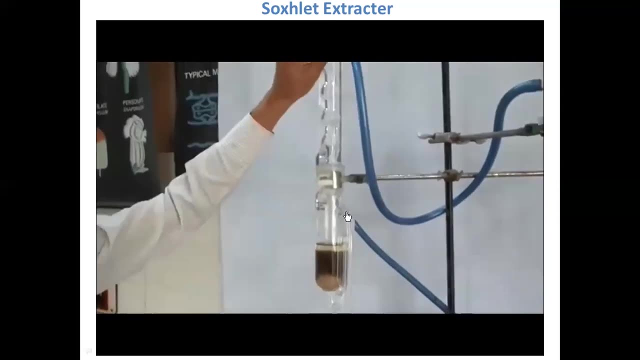 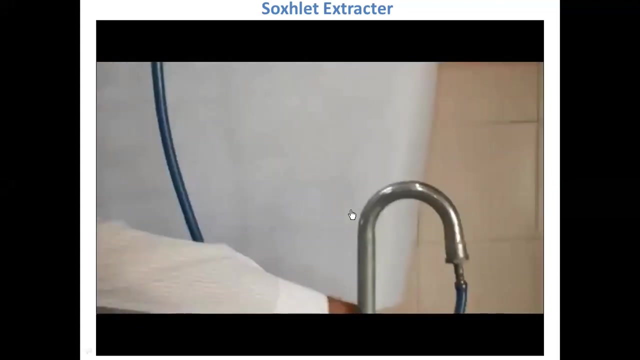 So water will be coming from the bottom and it is going out from the top, So you can see water flow. You can see water flow, So water passing should be continuous. You should not stop the passage of the water, because this would be a continuous process. 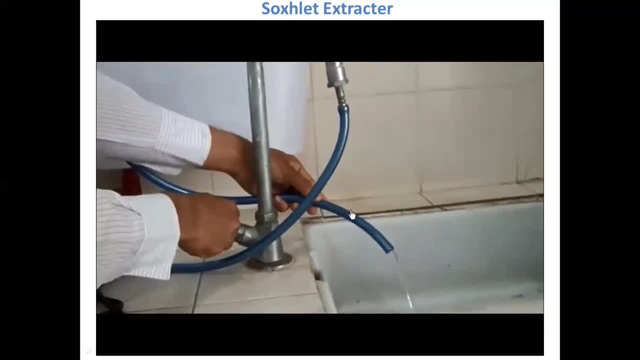 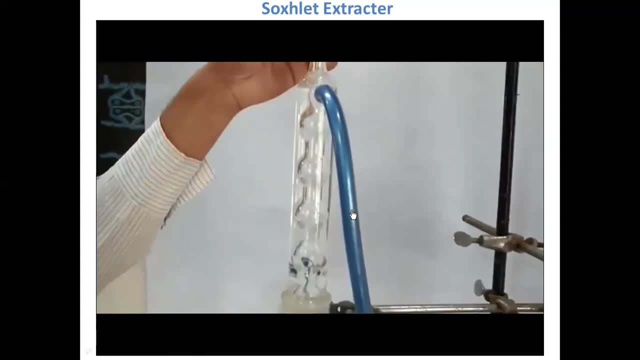 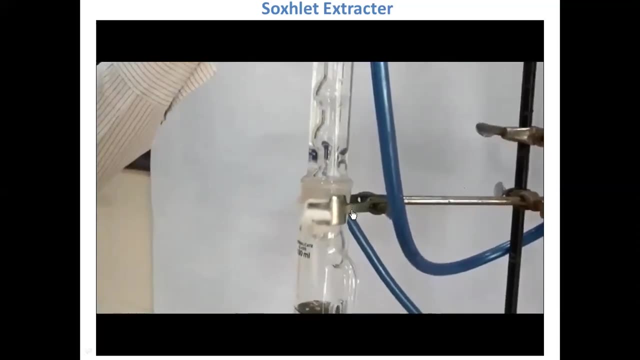 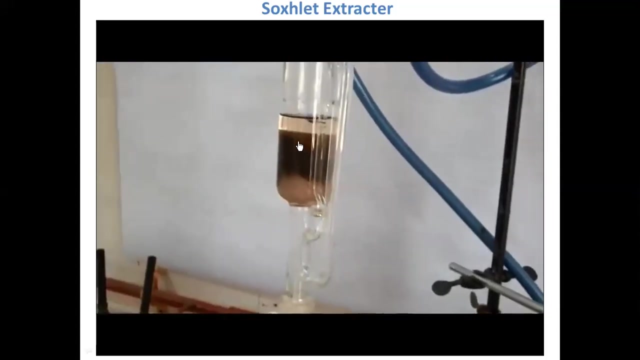 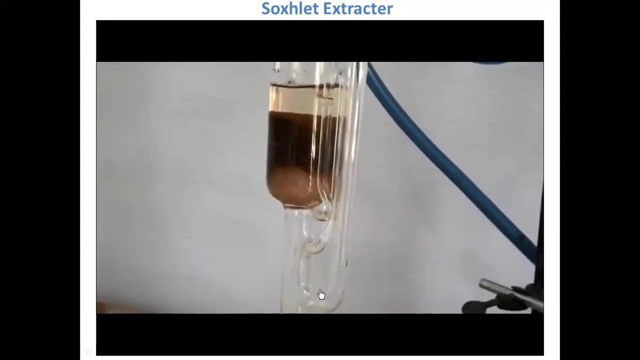 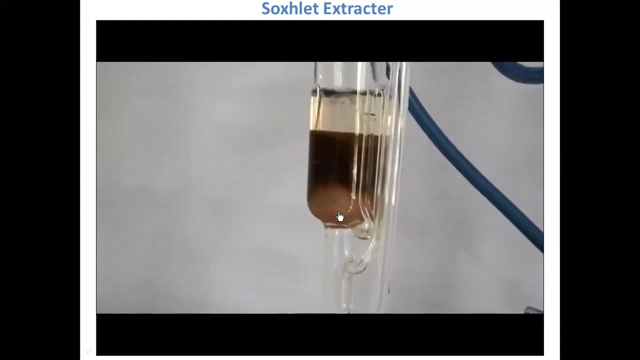 If water flow is stopped, there will be chances of damaging the instrument, damaging the operators. Therefore, the flow of water must be continuous. So the solvent has been added to the sample compartment. The round bottom flask has been fixed If you wanted to get the dilute solution. 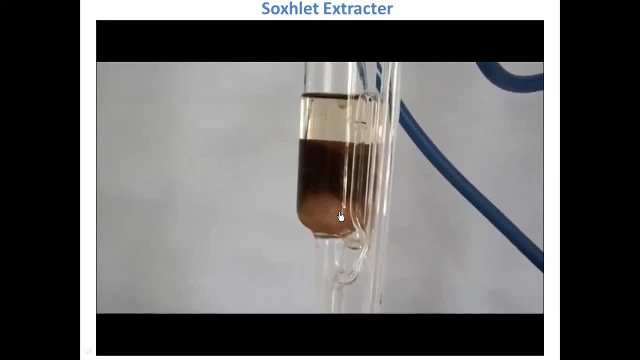 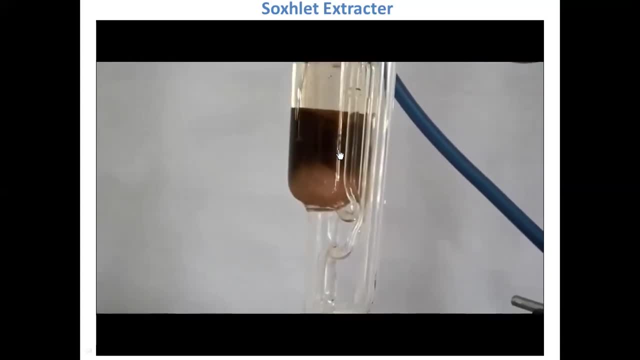 the solvent reservoir can also be contained in the soxhlet, So the solvent is contained with several milliliters of the solvent, as I told in the beginning. So now the sample is ready to perform the extraction process. So what should be the next procedure? 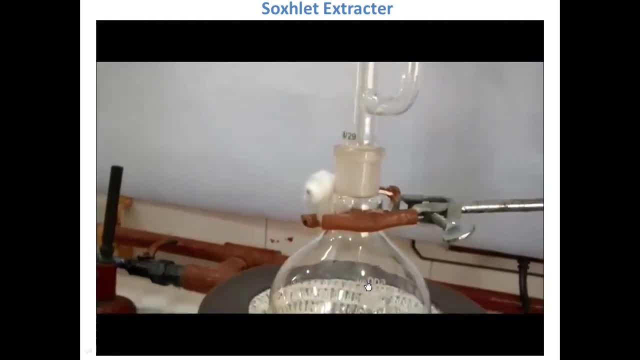 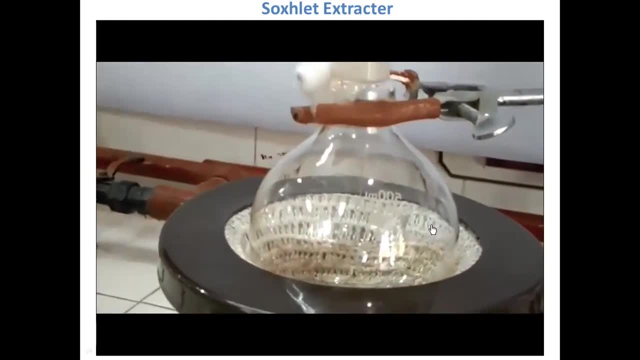 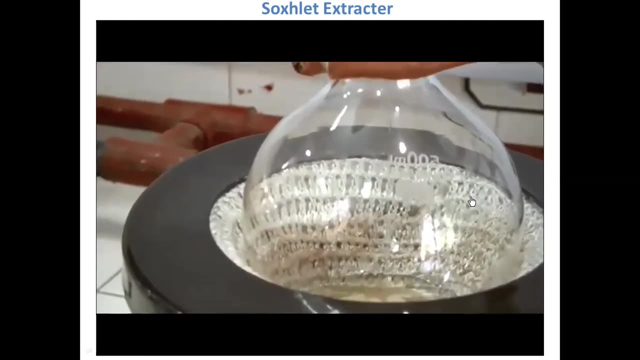 So you have to switch on the instrument. After switching on the instrument, the heating up of the solvent will be taken place, So solvent vapors are produced. Then those vapors are going to be converted into droplets by the condensation process. 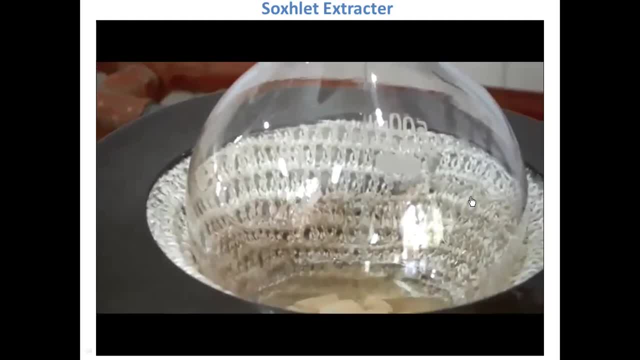 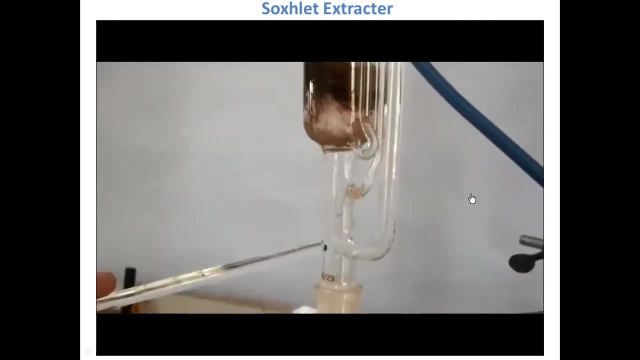 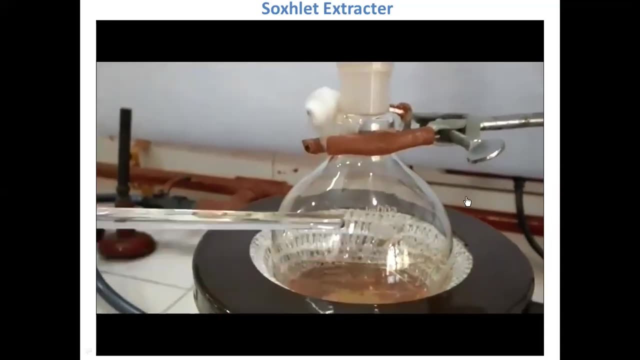 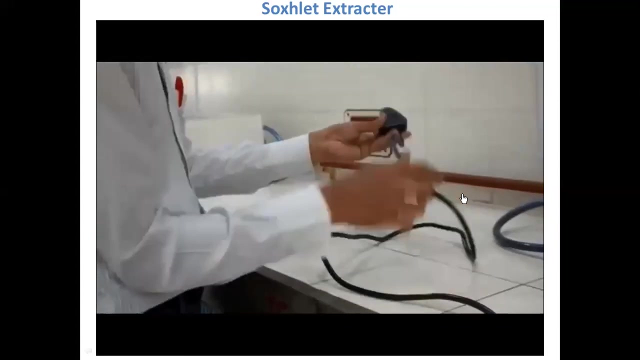 And the condensed liquid will be interacting with the solutes present in the sample. So you can see the moment here, how the solution coming back to the solvent reservoir, So from the solvent reservoir, droplets are obtained by heating, And this heating will be done by the influence of a liquid. 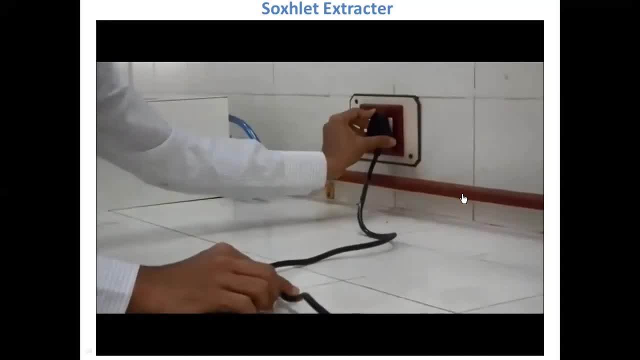 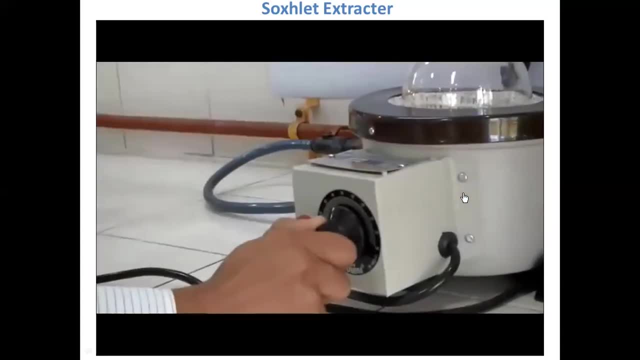 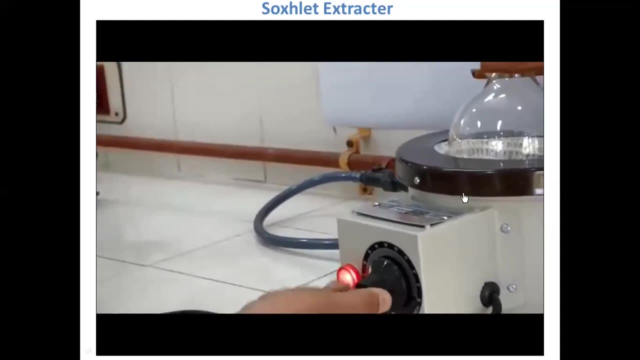 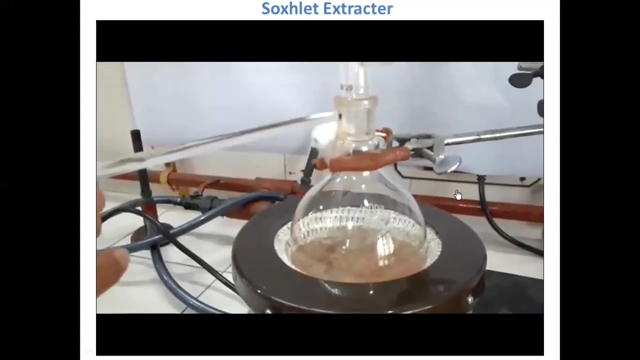 It's a telephone, So we switch on the solvents here to allow the solvents to heat and scalp off So you can see how the solvent is starting to heat and will complete the들曬an happen. this should allow the solvents to heat up faster than we do afteryez. 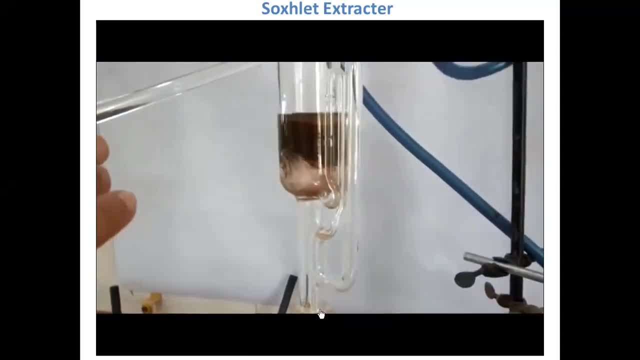 when the solvents are discharge. Once the power is switched on, the solvent will be getting heated. Now the heated solvent will be converted into vapers, because it is volatile, tube vapors from the solvent reservoir, because the solvent has been converted into vapor and the 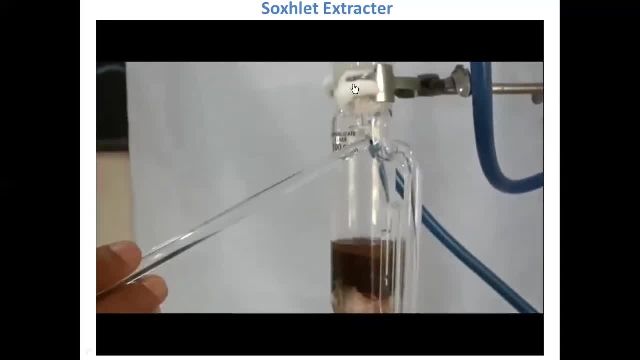 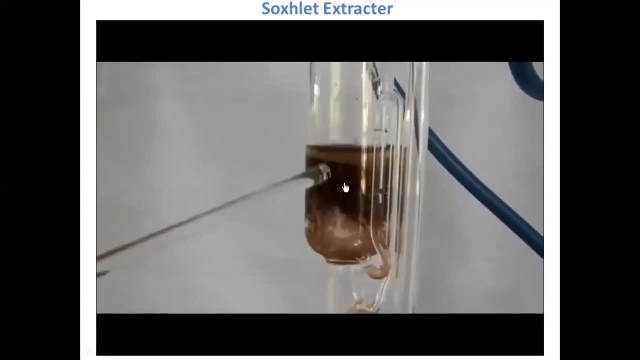 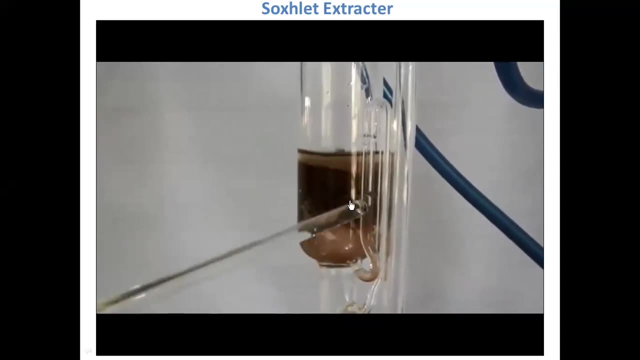 vapors through this vapor tube will be going up and it will be condensed back by means of the condenser and it will reach the sample. in this sample compartment, the solvent will be interacting with the solute present in the sample and the extract. extract, when the level of the liquid 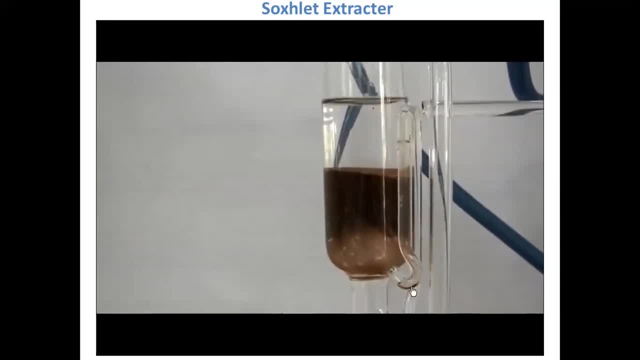 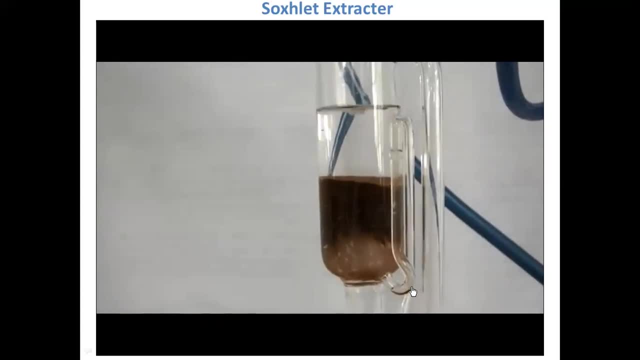 increase. the extract will be reaching back to the solvent reservoir. so the sample components are the analyte components present in the sample are dissolved in the solvent, which is passed into the sample compartment by vaporization process followed by condensation process. they will be reaching the solvent reservoir that is present in the round bottom. 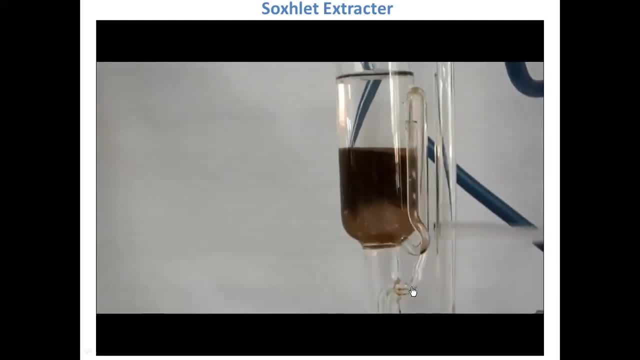 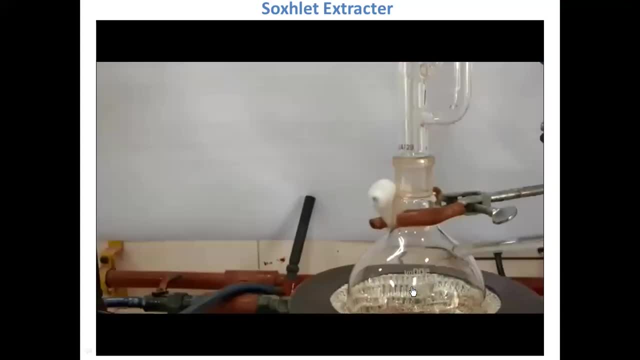 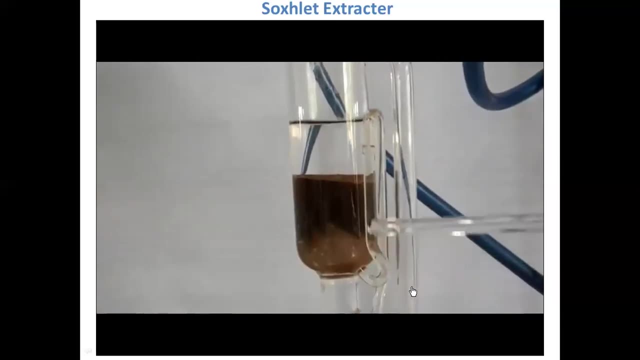 flask. so the round bottom flask is uh. at the initial stage it will be containing only solvent and once the extraction process is over, the round bottom plus will be containing not only the solvent but also the analyte. whichever the solutes present in the sample are having greater 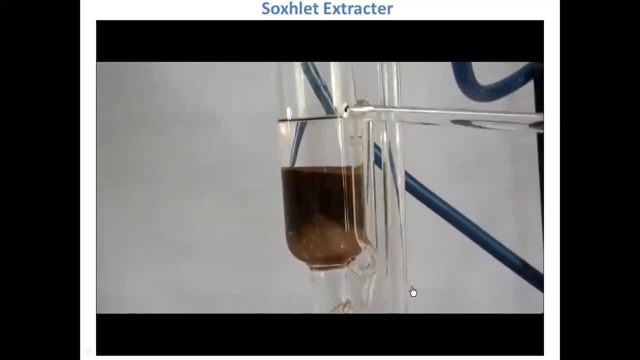 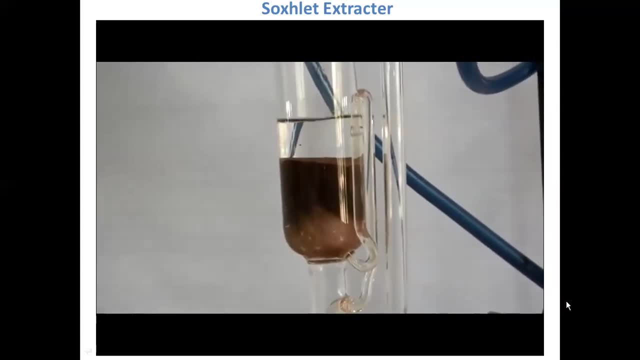 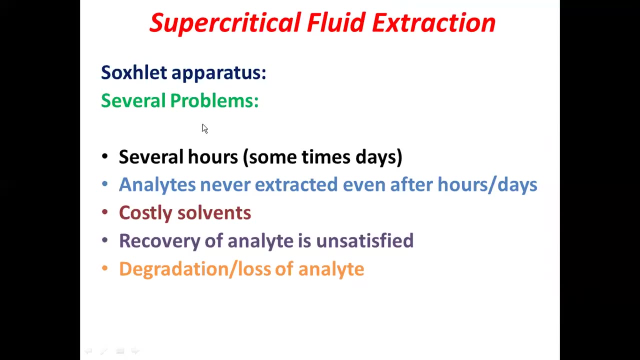 selectivity- to get dissolved in the solvent they are going to be dissolved or they are going to be extracted into this particular solvent and therefore they are extracted into the solvent which is present in the round bottom flask. so this is about the sachlet extraction procedure. so there are several problems while performing the extraction by sachlet operation. sachlet operation. 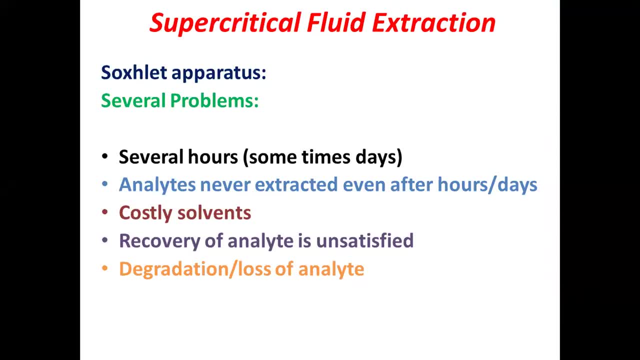 or sachlet extraction is not stipulated to lower interval of time. several days may be required. sometimes several days may be required in order to complete the extraction process. you can see in our laboratory some people will be keeping for the extraction, at least for a couple of days. so even you perform the extraction for a couple of days, the extraction efficiency will not. 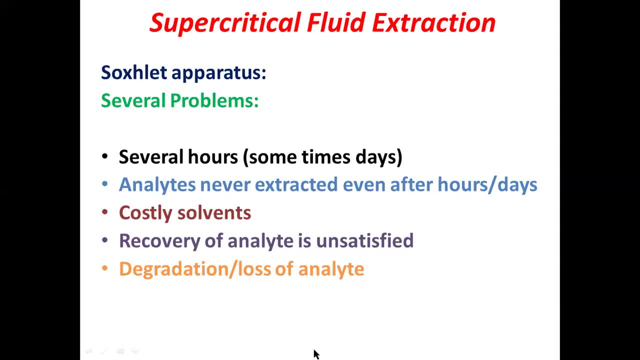 be 90 percent. even so, even if you do the extraction for several hours or several days, the analyte is not going to be extracted more efficiently and the solvent we are going to use may be toxic or it may be harmful. and the solvents may be very costly and the recovery 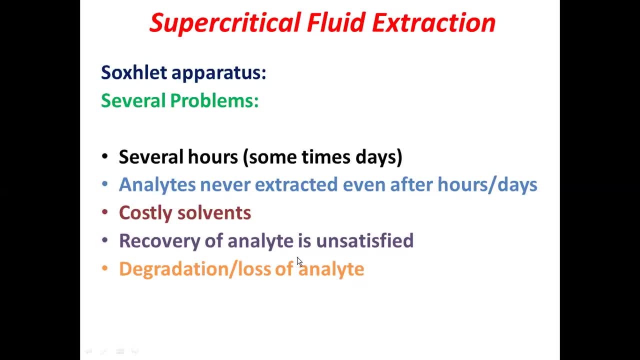 of the analyte will be unsatisfactory. so we cannot recover the analyte satisfactorily because we are going to perform, uh, the extraction with the aid of it. so loss of analyte or degradation of the analyte, these are the common problems we can see. 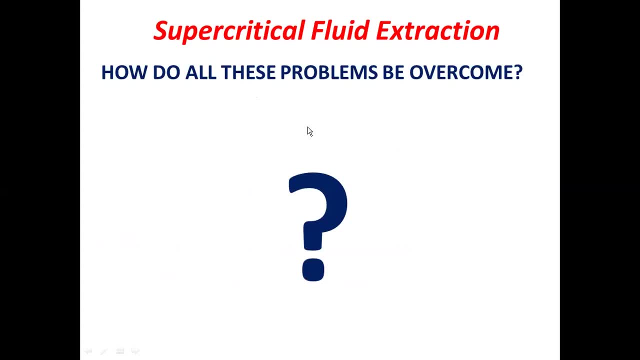 by performing the sachlet extraction process. how to overcome all these problems? we need to recover the analyte satisfactorily, analyze should not undergo any degradation or loss. we must use a low cost solvents and the solvents must be innocuous, they must be harmless, they must be non-toxic. 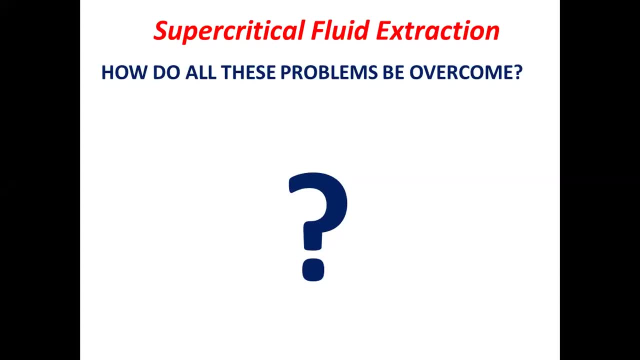 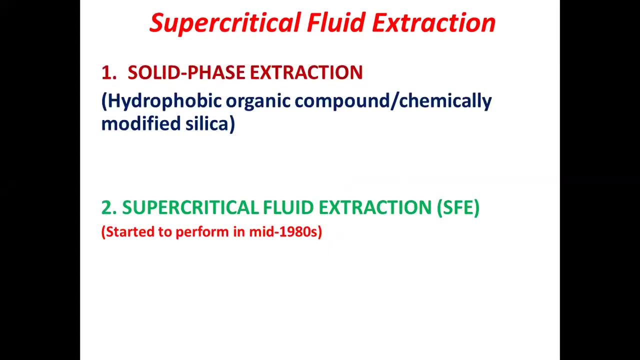 and the quantitative recovery of the analyte must be possible. these are the requirements in order to consider any extraction technique. so the problems of sachlet extraction, how they are going to be overcome, these limitations can be overcome by using two important extraction techniques. one is going to be solid. 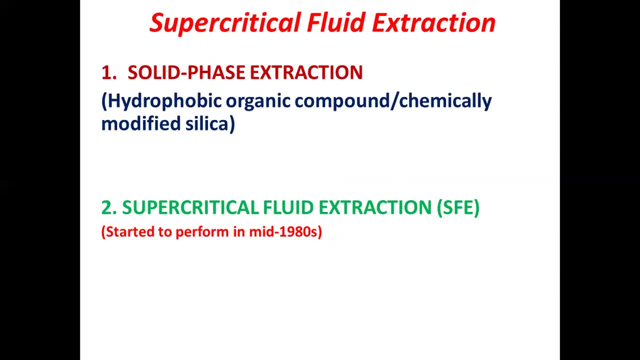 phase extraction technique by using hydrophobic organic compound such as chemically modified silica or silica as an adsorbent or the surface of the adsorbent. the solute molecules are going to be absorbed- absorbed and thereby the extraction is possible. and the second one is a very popular 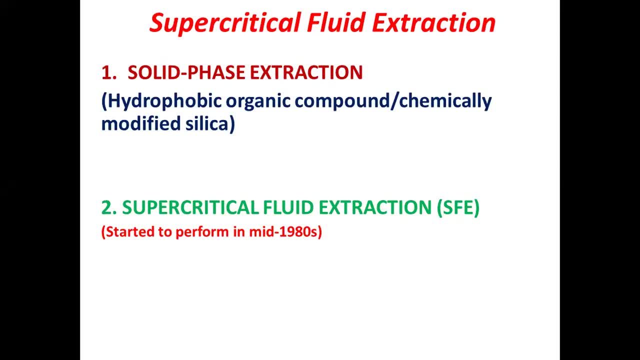 technique, which is known as supercritical fluid extraction technique, in which the extraction of the analyte is possible by means of a supercritical fluid because it is going to exhibit intermediate properties such as higher density, higher, lower viscosity and higher diffusion coefficients when compared to those of 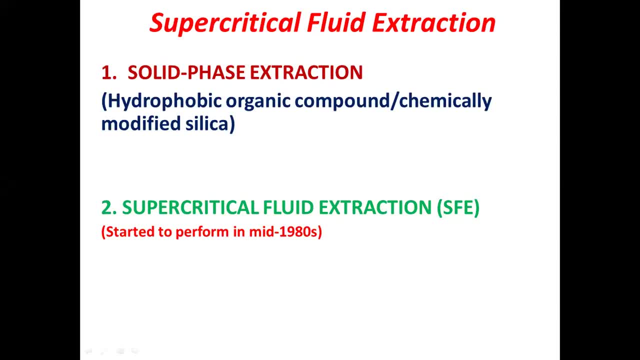 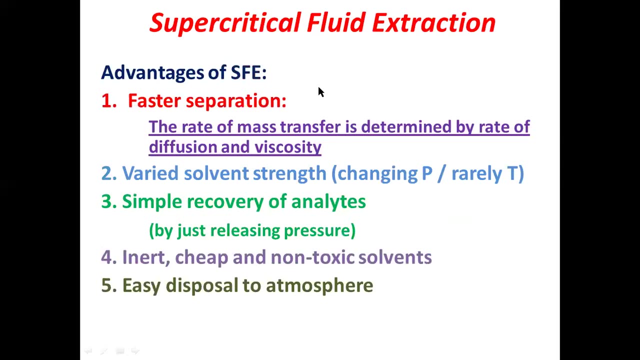 gaseous or liquid substances. so these supercritical fluids were invented in the year 1970s and the supercritical fluid extraction technique was developed in the year 1980. so because of the advantages of faster separation, in which the rate of mass transfer is determined, 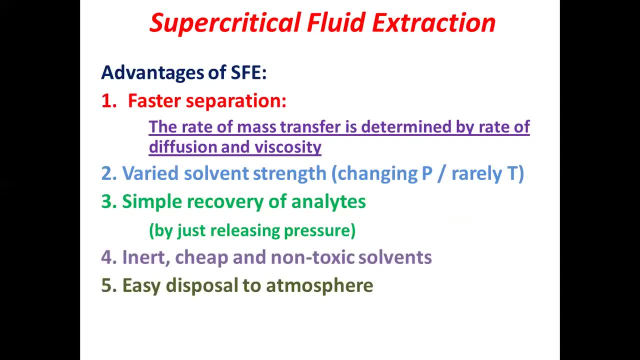 by rate of diffusion and viscosity. as i told you, the diffusion coefficient of the supercritical fluid will make the dissolution of the solute more comfortably and the separation will become possible because of the viscosity of the supercritical fluids. so faster separation is possible because of the varied solvent strength and that is also due to the diffusion and viscosity. 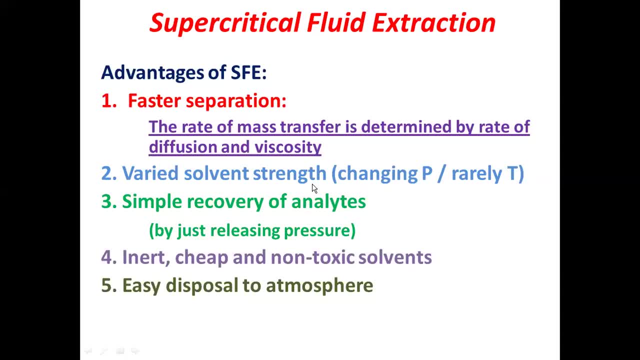 and this varied solvent strength can be obtained by changing the pressure, but very rarely by changing the temperature. the supercritical fluids are always advantageous in order to succeed the extraction process and the recovery of the analyte by just releasing the pressure is very simple while performing the supercritical fluid extraction. therefore, this is also one of the 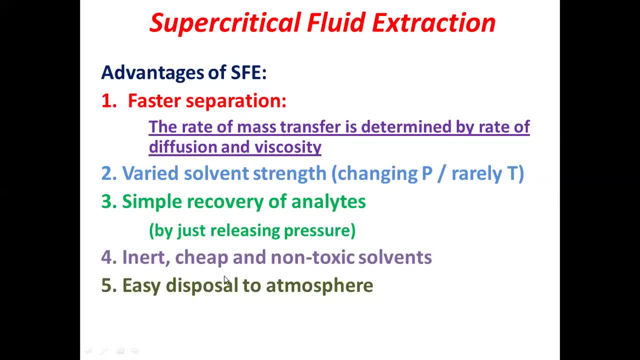 important advantages of performing supercritical fluid extraction and the supercritical fluids. if you take supercritical ammonia, supercritical carbon dioxide or supercritical nitrous oxide, whatever it is, they are inert, they are highly inert. they are not harmful, they are cheaply available, they are non-toxic. so 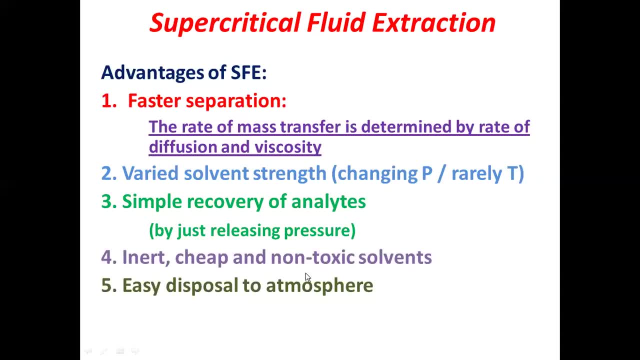 because of inertness, a cheaply availability and non-toxic property of these solvents, the extraction procedure will become environmental friendly and once the extraction procedure is over, we can easily dispose of these supercritical fluids into the atmosphere. so these are the important advantages of supercritical fluid extractions which are performed by using supercritical fluids. 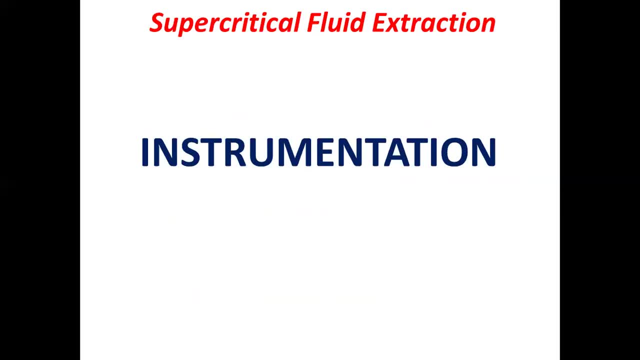 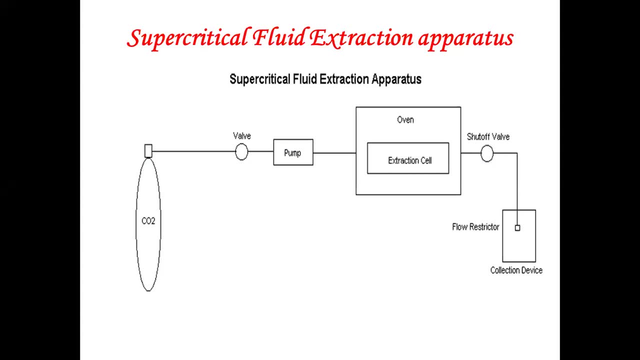 let's move on to the instrumental part, how we are going to perform the supercritical fluid extraction. this is going to be the instrumental schematic which can be used while performing supercritical fluid extraction. so, as you can see here, a supercritical fluid tank will be used and that will be connected to a wall entry wall. this is called as the entry wall and 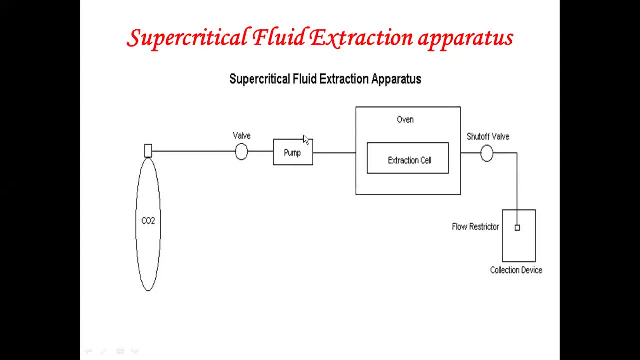 this entry wall is connected to a syringe pump. this syringe pump is required to create the sac authorized is needed to be created and this is the extraction cell. and this extraction cell is placed in a thermostatically controllable one because one is required to adjust the temperature in order to attain the supercritical fluid. 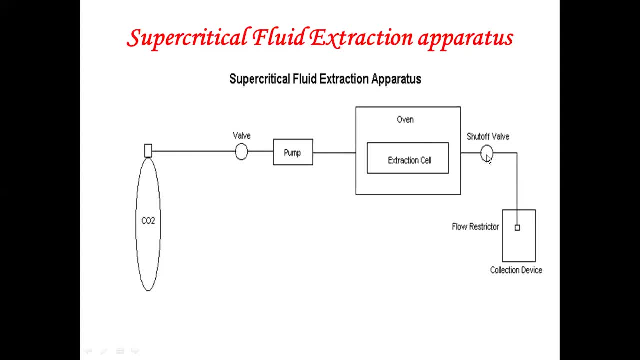 state and there will be a set of wall. this is the entry wall. this is going to be the set of wall. this is a flow restrictor. this flow restrictor will be a capillary tubing, will be having a length from 10 to 20 centimeter, 10 to 20. 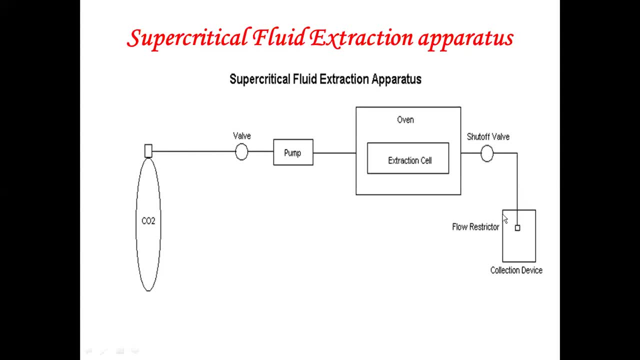 centimeter length. this capillary tubing will be having- and this is a collector, divisor, collector, flask collector class. so these are the components. supercritical fluid carbon dioxide will be connected to a wall, followed by a syringe pump, and this syringe pump is connected to the extraction cell. this extraction cell is: 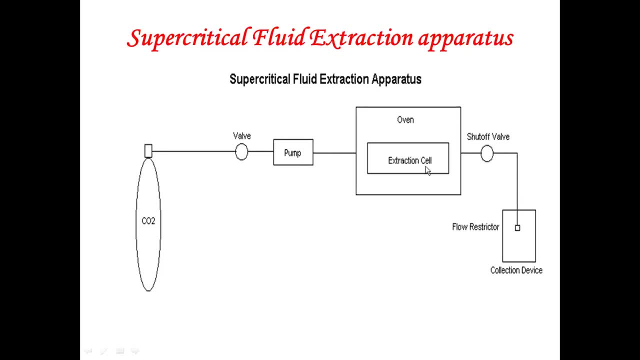 placed inside the woven in order to heat the extraction cell, you I'll to attain the supercritical fluid state for the solvent at the extraction substance and the set of wall will be available soon after the extraction cell. from the set of wall there will be a capillary flow restrictor and which can 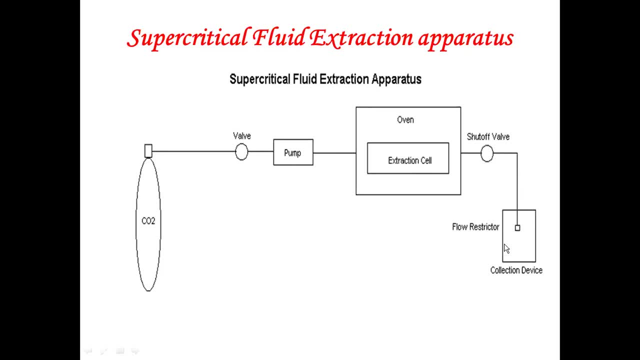 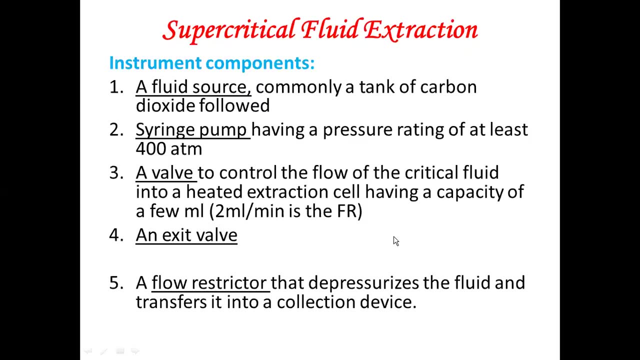 be immersed or penetrated into the collection device, and this collection device will be having a solvent in which the dissolution of the analyte can be expected more satisfactorily. okay, so, as you can, as you saw in the diagram, you can see that this is the capillary fluid state and this is the 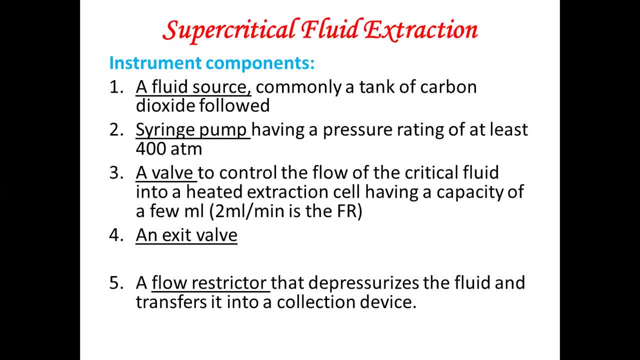 dijla Curiosity. Solid diagram. fluid source is commonly supplied from a tank. more commonly, if the supercritical carbon dioxide carbon dioxide will be filled in the diagram. a fluid source is commonly supplied from a tank. more commonly, if it is supercritical carbon dioxide, carbon dioxide will be filled. 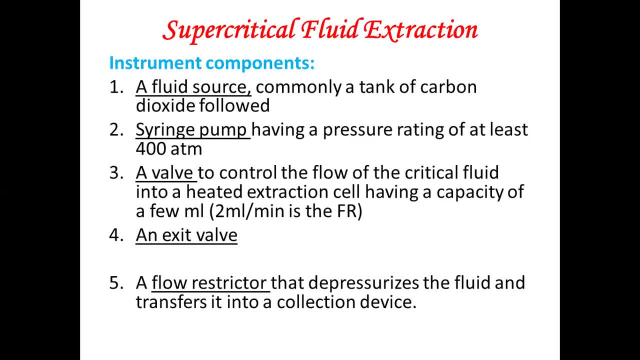 in the tank. if it is ammonia, ammonia is going to be filled there. if it is net ämän air, it is going to be filled over there and the syringe pump will be having a pressure rating of at least 400, which will be the capacity in order to adjust the pressure. a wall to control the flow, because we need to adjust the flow rate optimally at 2ms from sound rate. 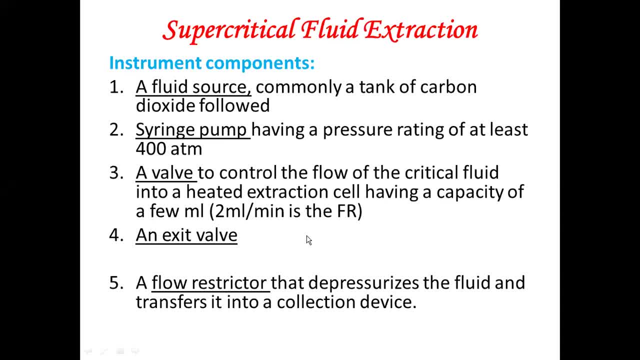 endra per minute during the extraction process. so valve is used to control the flow rate, an exit wall in order to give the exit for the components separated in the extraction cell, and the flow restrictor is utilized to depressurize the system because pressure is above the critical pressure. temperature is above the critical temperature. we need to depressurize. 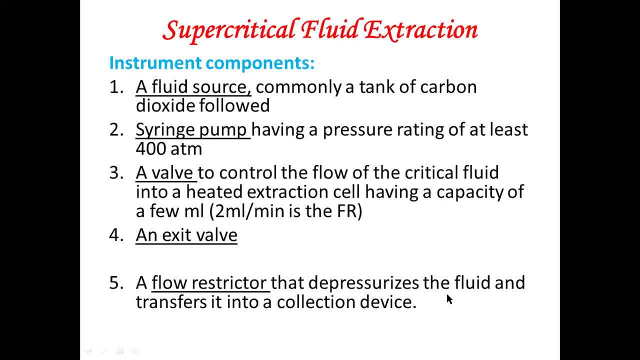 in order to make the fluid to be escape to the atmosphere. therefore, all those separated solutes must be entered into the collection device, and it is containing the solvent in which the analytes are going to be dissolved, so a fluid source containing the fluid, such as carbon dioxide, ammonia, nitrous oxide. a syringe pump will be used to create the pressure. 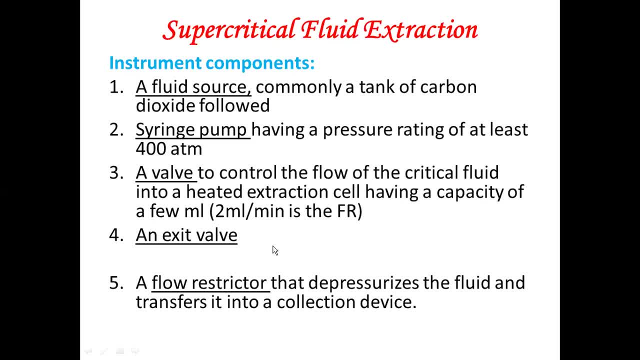 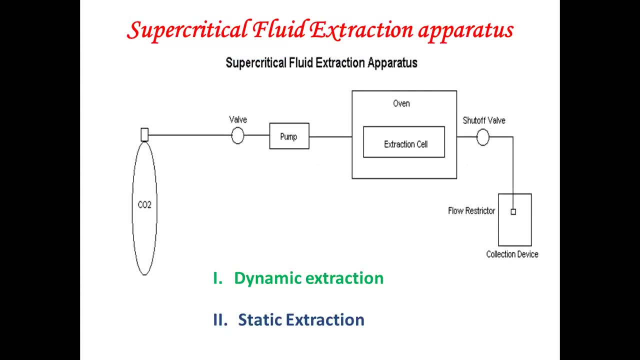 a wall to control the flow rate of the fluid and the exit wall to give the access to the components which are separated in the extraction cell. and the flow flow restrictor is used to depressurize the system. so, while using this instrumentation, the extraction will be done. 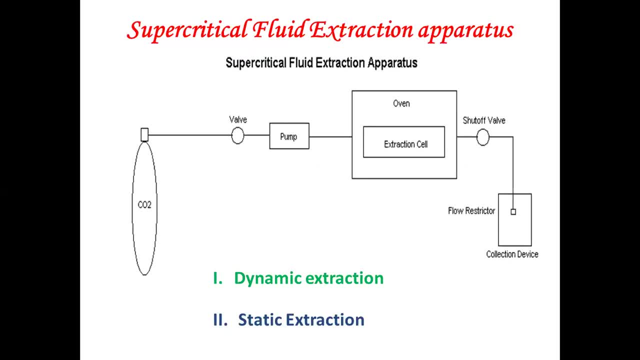 in two ways. the supercritical fluid extraction will be done in two ways. what are those two ways? dynamic extraction and static extraction. dynamic extraction and static extraction: what is the difference between these two? the extraction principle remains the same. supercritical fluid will be the solvent into which 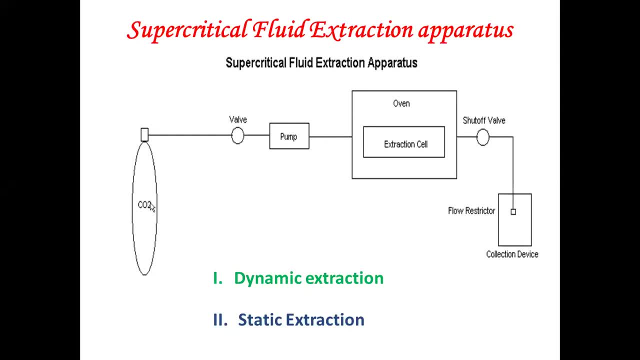 is going to be extracted, so that is going to be supplied by means of a tank. so then, what is the difference between dynamic extraction and static extraction? usually, the extraction procedure is initiated by filling the extractions. we can remove this extraction cell out to take the extraction cell. 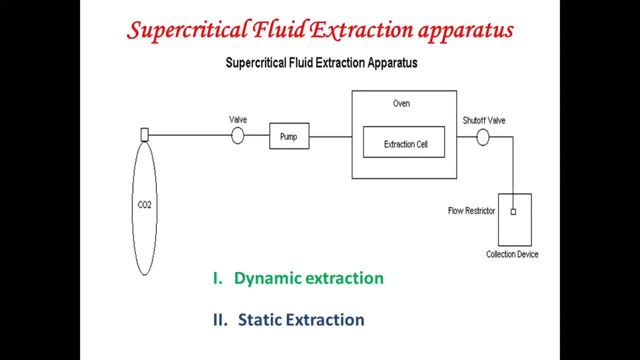 out, introduce the sample solution in this extraction cell. sometimes even we may take a solid samples directly from the extraction cell and then we can extract it from the extraction cell directly in the extraction cell. or liquids we can take whatever it is. you take the sample in the 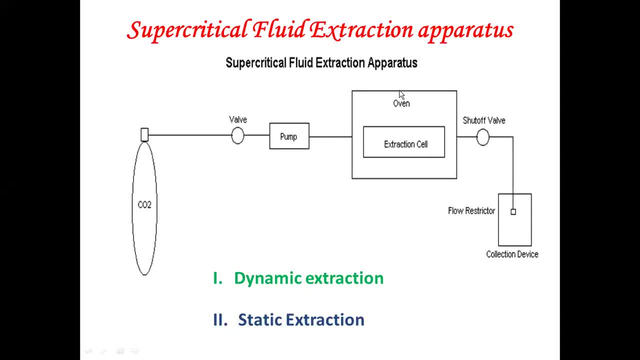 extraction cell. keep the extraction cell inside the o1. make sure that it has been connected to the pump terminal of the capillary from the pump. okay, next is we have to perform the extraction. you create a continuous flow of carbon dioxide at an adjusted pressure, in such a way that gaseous carbon dioxide has been converted into. 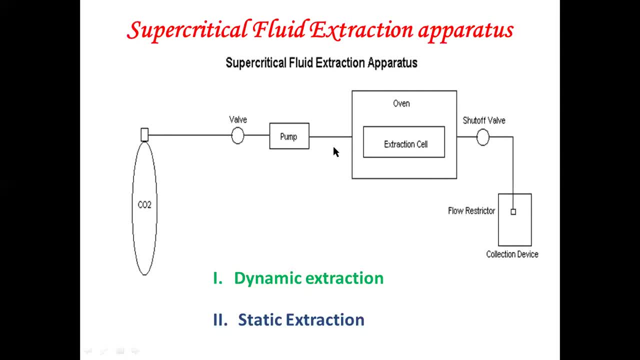 supercritical carbon dioxide and in that particular state the supercritical carbon dioxide is entering the extraction cell. in the extraction cells analyzed present in the extraction cell in the sample. they are going to be extracted by the carbon dioxide because carbon dioxide is present in its supercritical fluid state. 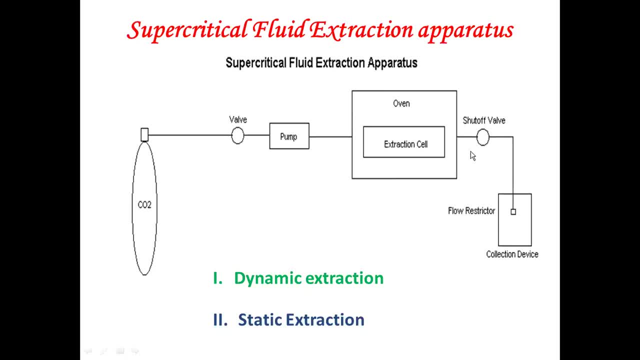 and during the extraction process, the set-off wall- here you can observe here set-off wall is opened always- is opened always. the set-off wall will not be closed during the extraction process. the extraction process will be continuous during the extraction, the set-off wall will not be closed. 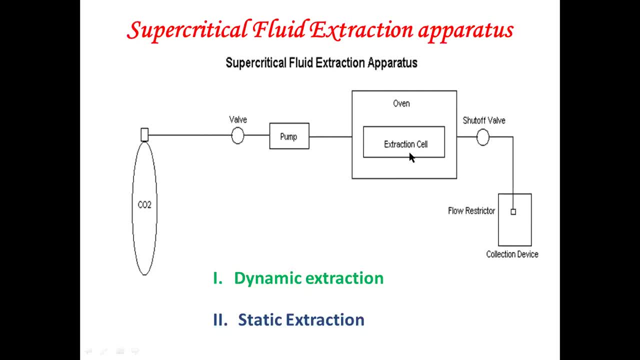 will be opened always. so, whatever the analyte getting extracted into carbon dioxide is continuously in motion and it will be reaching the collection device through the flow restrictor. through the flow restrictor. this is called as dynamic extraction. so dynamic extraction means the set of wall between the flow restrictor and the extraction. 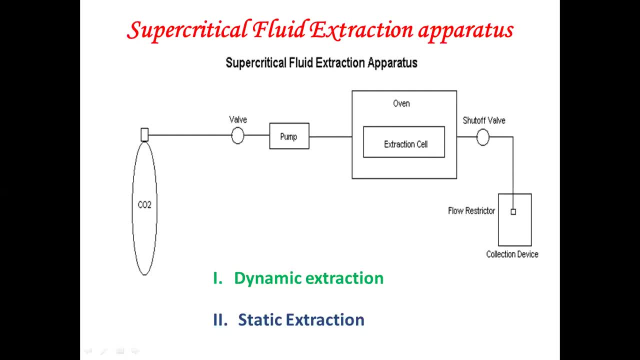 cell will be opened throughout the extraction process. during the duration of the extraction process, the set of wall between the extraction cell and the flow restrictor will be opened, so the movement of the analyte will be continuous. whatever the analyte moving through this capillary or the flow restrictor will be reaching the collection device and this collection device. 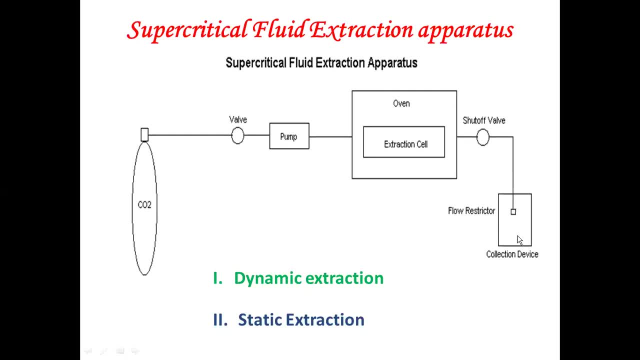 is containing the solvent, so analyte will be dissolving in this collection device or in this solvent present here. flow restrictor is a capillary where the pressure is adjusted in such a way that the supercritical flow fluid state for the carbon dioxide is disturbed, So the gaseous carbon dioxide will be escaped. 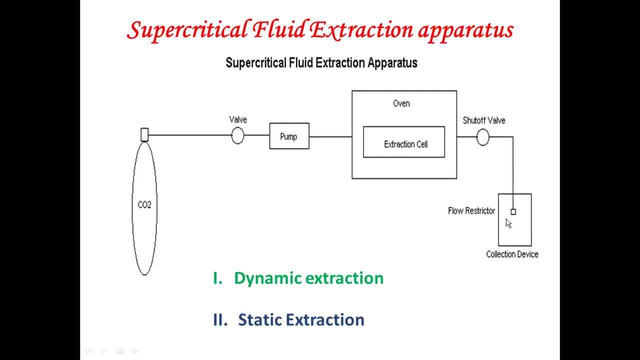 to the atmosphere and only analyte will be reaching the collection device. so the analyte will be dissolving in the solvent present in the collection device. This is called as dynamic extraction. In static extraction, the set off wall between the extraction cell and the flow restrictor will be closed for a period of time. will be closed for a period. 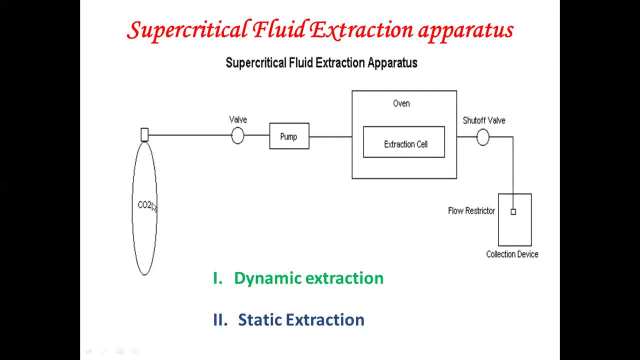 of time during which the interaction between supercritical carbon dioxide and the analyte present in the extraction cell will be taken place. Static means closed. static means closed, So set off wall will be closed. set off wall, which is present in between extraction cell. 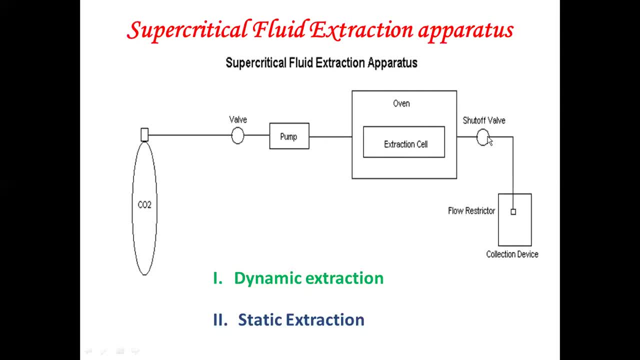 and the flow restrictor will be closed for a certain period of time, during which the extraction is stopped. After some interval of time, this set off wall is going to be opened and the solutes are procured in the dynamic method. This type of extraction is called as static extraction. 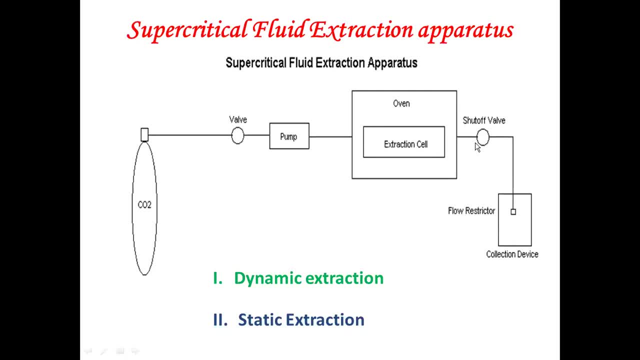 So in the dynamic extraction, throughout the extraction duration, the set off wall will be opened. In the static extraction, for a period of time the set off wall will be closed, then it is opened. So this is the way of the anatomical collection, The analytical process in the collection device. 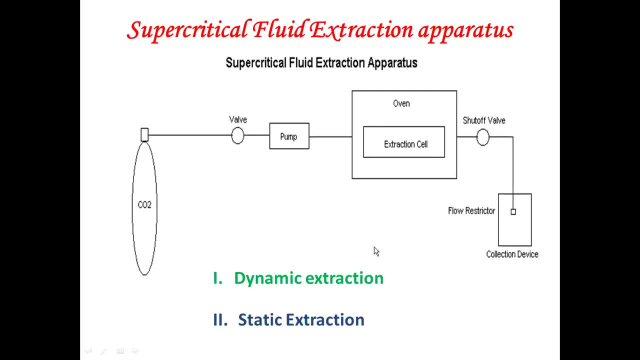 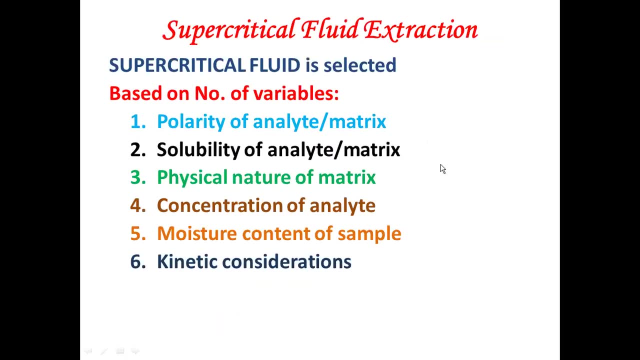 is the same in both the techniques. This is how we can differentiate dynamic extraction from static extraction. What are the choices of supercritical fluids, What are the substances we can use them as supercritical fluids and what are the requirements? Based on certain variables, we'll be in a position to choose the supercritical fluids. 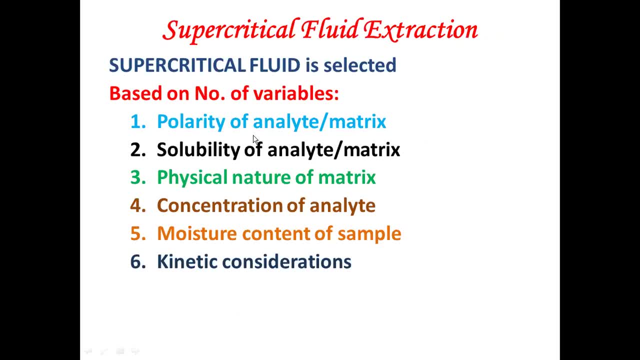 importantly the polarity. here, as i told while explaining the liquid, liquid extraction or solid phase extraction: like dissolves like or like attracts like. principle holds good. in order to increase the separation efficiency, unlike here- also the polarity of the analyte or polarity of the matrix with respect to the supercritical fluid must be matched. 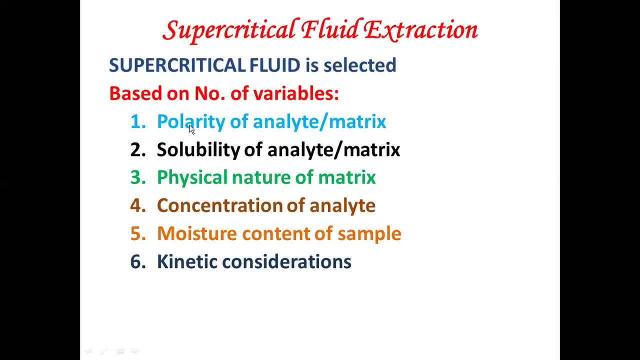 such a supercritical fluid will be chosen means the polarity. if analyte is polar, polar supercritical fluid is not going to become responsible to hold the polar analyte and the non-polar supercritical fluid will not become responsible to hold the non-polar analyte. 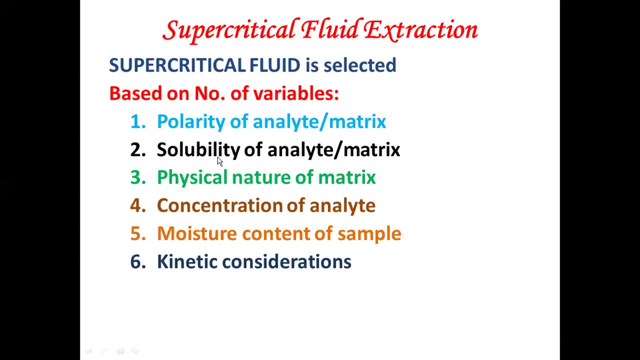 or vice versa. diffusion coefficient of the supercritical fluid. we must concentrate because solubility is very important here. the analyte of the matrices, whatever present in the sample, must be easily soluble in the supercritical fluid. and not only the dissolution but also nature of the matrix. 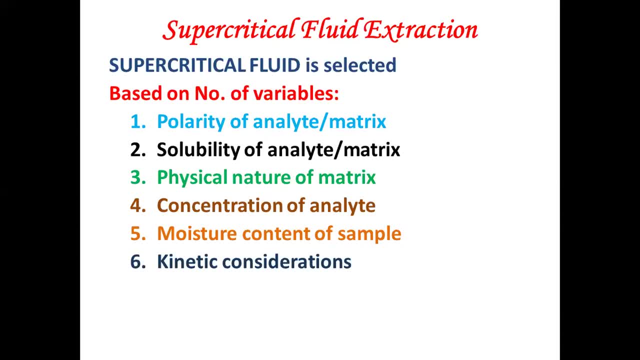 what kind of the matrix present in the sample. that should not interfere during the extraction procedure or the separation of the analyte from the matrices by this supercritical fluid. extraction supercritical fluid should not create any interference from the matrix and the solution after extraction is over must be highly concentrated, so moisture content of the sample is. 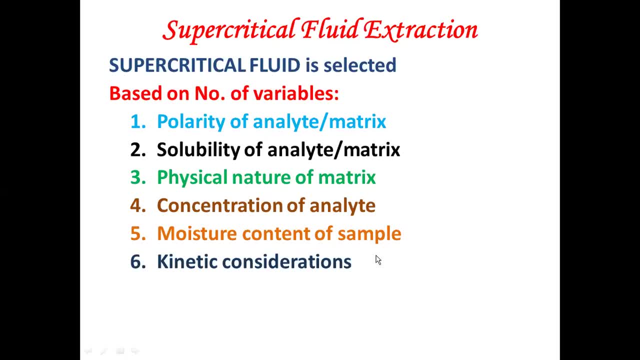 also very important. so if we are going to use some hydrophobic supercritical fluids, moisture is not going to be removed. so such a supercritical fluid we need to consider and some other kinetic considerations because i told you, kinetic energy by the movement of the molecules is going to be larger when compared to 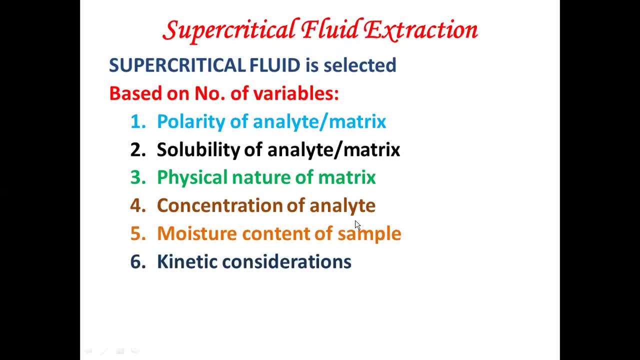 the intermolecular forces of energy. therefore, these kinetic considerations can also be considered. so these are the requirements while choosing the supercritical fluid. first one: polarity should be matched, solubility must be satisfied. physical nature of the matrix must be seen carefully. concentration of the analyte must be. 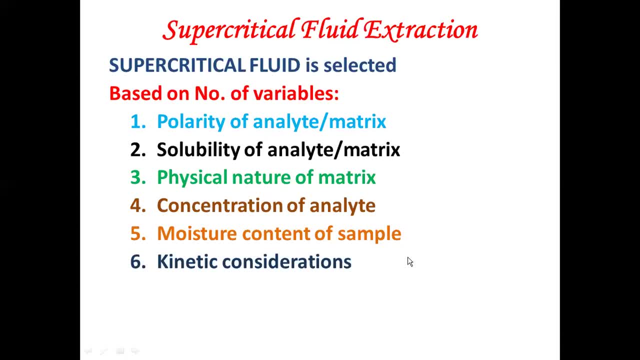 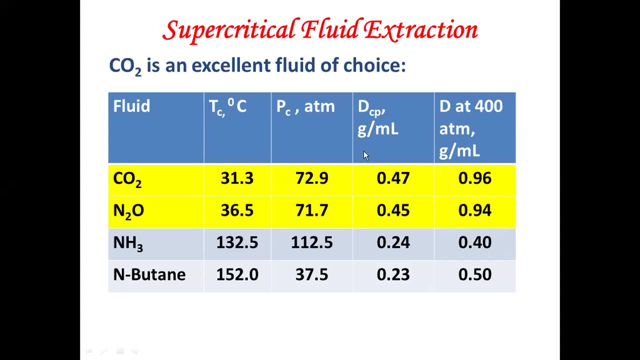 appropriate and adequate moisture content of the sample. we must have the knowledge, and other kinetic considerations must also be considered. carbon dioxide is an excellent supercritical fluid and which is used in more than 80 percent of the supercritical fluid extraction, either alone or by mixing with some modifiers, i can 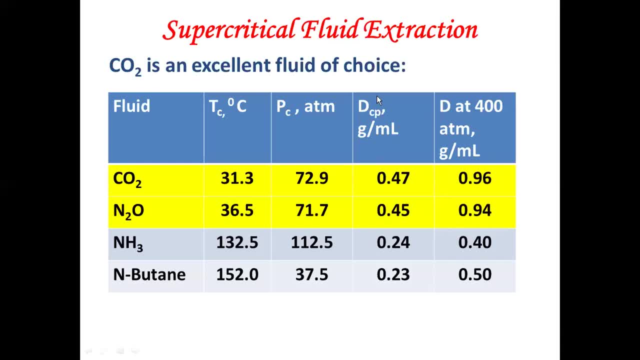 tell you about the modifier. so what is the meaning of modifier and so on, why this carbon dioxide is used. i have presented here a table uh showing the critical temperature, critical pressure, the density at critical pressure and density at 400 atmosphere for carbon dioxide, nitrous oxide, ammonia and n-butane. so these four are used as supercritical. 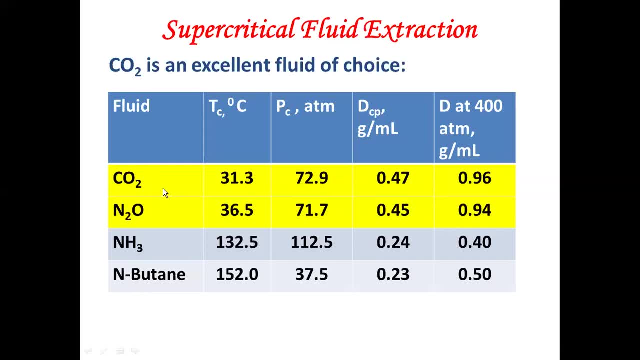 fluids. if you look at the critical temperature of carbon dioxide, 31.3 degrees celsius, and the critical pressure will be 72.9. atmosphere density: 0.47 gram per ml. similarly, nitrous oxide, you can see 36.5- close to 31.3, 71.7- very close to 72.9. 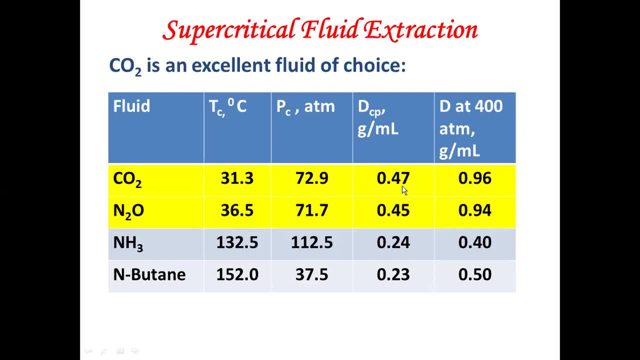 and even the density 0.45, almost similar to 0.47, a density at 400 atmosphere: 0.94. there is no much difference with 0.96, so i have made here yellow, because these two fluids can be commonly employed as supercritical fluids. 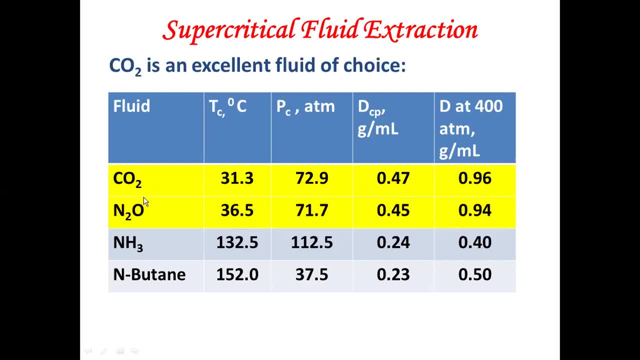 because the ability to make this carbon dioxide, nitrous oxide, to get converted them into supercritical fluids by just raising the temperature to 31.3 degrees celsius or 36.5 degrees celsius. so if you raise the temperature above 31.3, 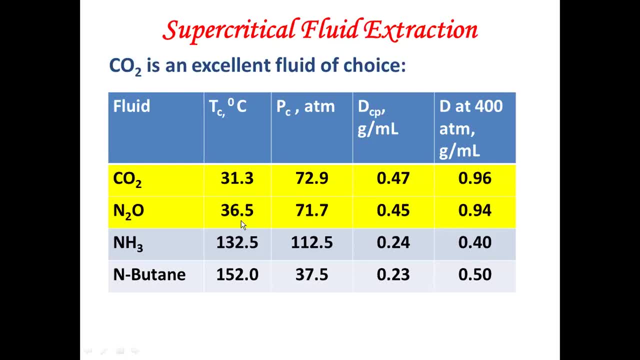 degrees celsius or 36.5 degrees celsius. carbon dioxide and nitrous oxide are easily converted into supercritical carbon dioxide or supercritical nitrous oxide and similarly, pressure, if you raise the pressure beyond 72.9 atmosphere or 71.7 atmosphere. 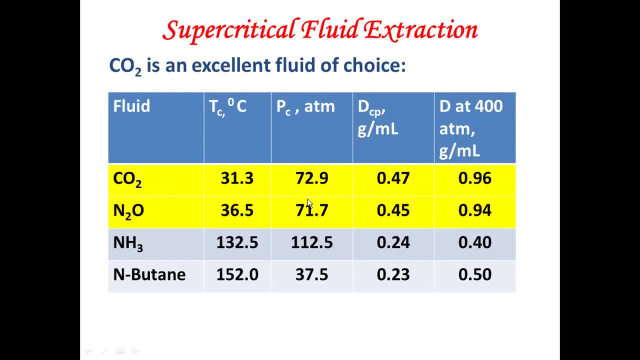 or the pressure will be above the critical pressure. therefore, supercritical pressure is very high. so if you raise the temperature to 32.5 degrees celsius or 32.5 degrees celsius, you are going to become responsible in order to convert these substances into supercritical fluids. 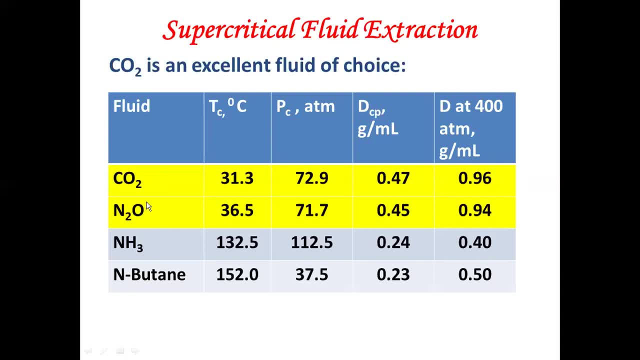 so the density is varied, but the same density when compared to nitrous oxide or carbon dioxide to each other: 0.47 or 0.45 at critical pressure or at 400 atmosphere. therefore, these two will become commonly used the supercritical fluids in order to perform the extraction by supercritical fluid extraction process. 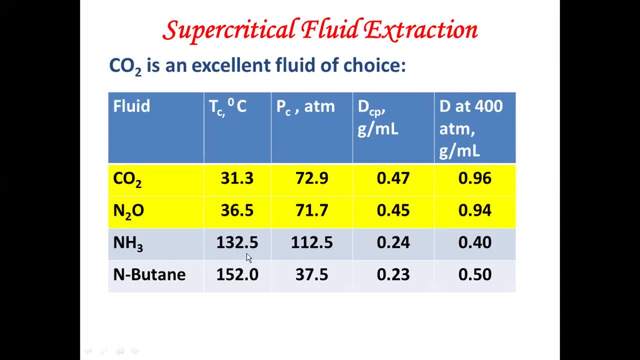 if you look at ammonia and n-butane, you look at the temperature- 132.5 degrees celsius and 152.0 degrees celsius here- but the density is very less. density is very less- 0.24 and 0.23- so density should be larger. larger density will be always advantageous. 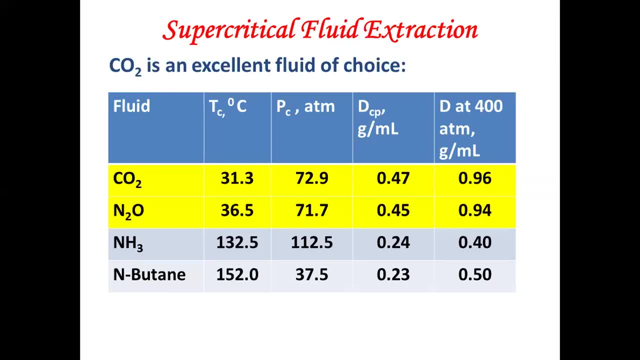 lower viscosity will be always advantageous. higher diffusion coefficient will be always advantageous. such a fluid will become adequately usable in order to perform the extraction by supercritical fluid extraction. so the uh, the chances of converting ammonia to supercritical fluid, is somewhat cumbersome when compared to conversion of carbon dioxide to. 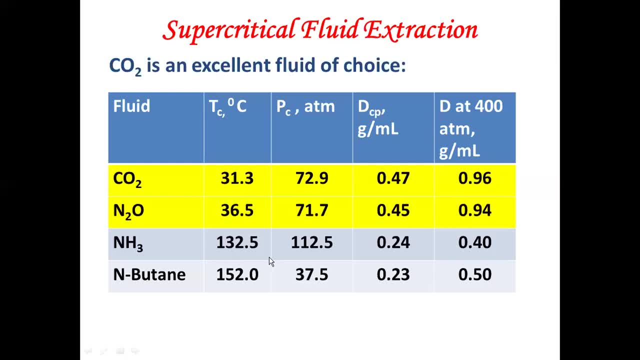 supercritical carbon dioxide because of the temperature here: 132.5 degrees celsius it is too far than the boiling point of water. 132.5 degrees celsius where you look at 31.3 degrees celsius, it is very close to room temperature because we are in the summer season. 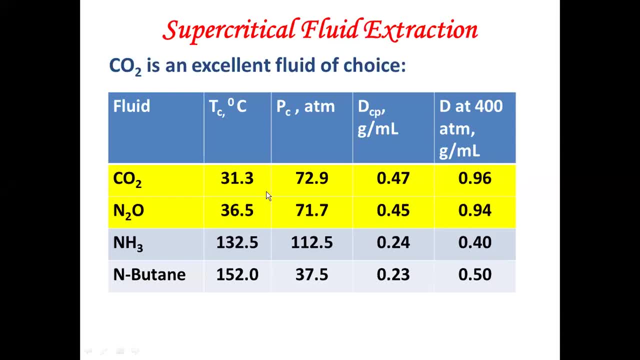 so temperature will be definitely greater than 30 degrees celsius. even it may be beyond 35 degrees celsius, so there is no any difficulty arise in order to adjust the temperature to either 31.3 degrees celsius or 36.5 degrees celsius, therefore attaining the supercritical fluid state for carbon. 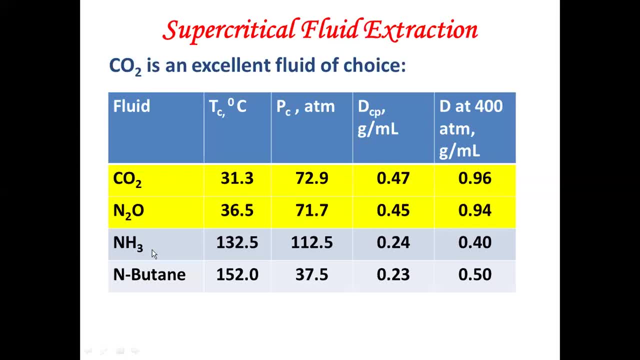 dioxide or nitrous oxide is very easy when compared to ammonia and n-butane, and ammonia and 10 are less commonly used because of their lower density when compared to carbon dioxide and nitrous oxide. so, because of these values, because of these order of magnitudes, supercritical carbon dioxide. 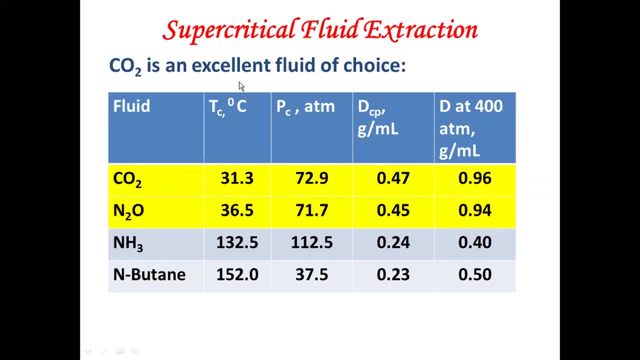 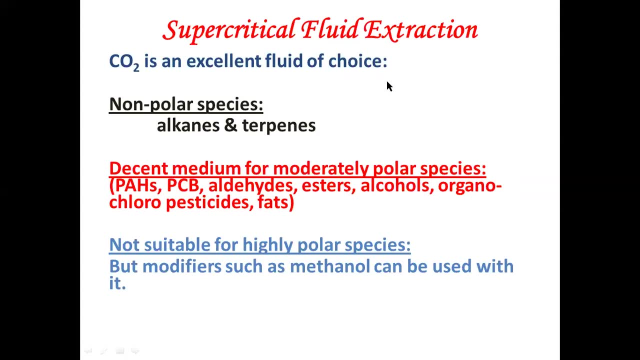 not only this, even n2o, nitrous oxide, can also be used as excellent fluids of choice in super critical fluid extraction operations. so let us look about the property of carbon dioxide, because carbon dioxide is used as a excellent fluid of choice in order to perform the super 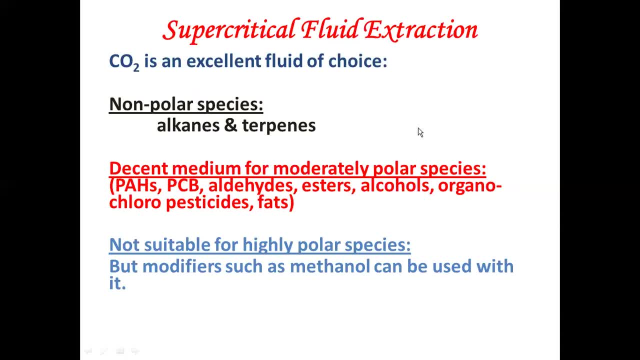 critical fluid extraction. if you look at carbon dioxide, it do not possess any dipole moment because it is a linear molecule: co2- c- double bond o towards the right hand side and c- double bond o towards the left hand side. it is a linear molecule, so, because of its linearity, do not possess any dipole moment and hence it is a non-polar species. 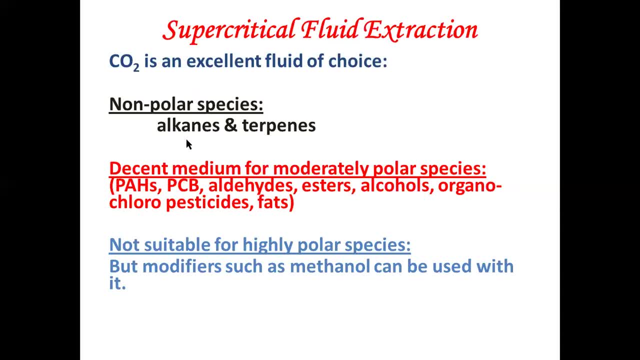 because of the non-polarity of carbon dioxide, all those non-polar alkanes and terpenes will be easily soluble in this supercritical carbon dioxide. therefore, this is an excellent fluid in order to perform the extraction of alkanes or terpenes, and it is also a medium for medium. 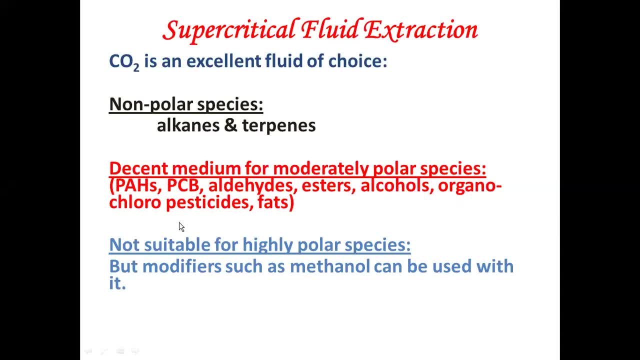 polar species, such as polycyclic aromatic hydrocarbons, polychlorinated biphenyls, aldehydes, esters, alcohols, organochloric pesticides, fats. but it is unsuitable for the separation of polar spaces because polar species do not show any interaction with the carbon dioxide. therefore, moderately polar 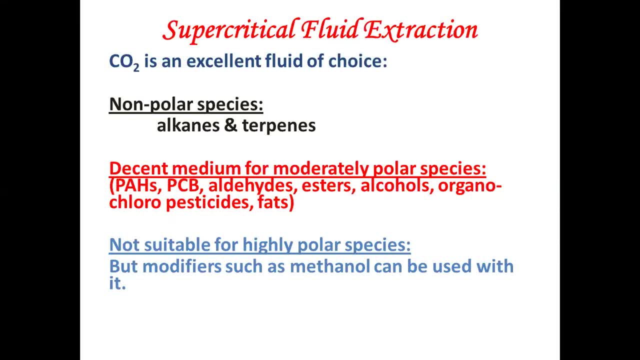 species can be easily separated from non-polar species and polar species when you use super critical carbon dioxide. so how do we overcome the extraction difficulty of species while using carbon dioxide as a fluid? so we can regulate the polarity of the carbon dioxide by mixing with the modifiers. 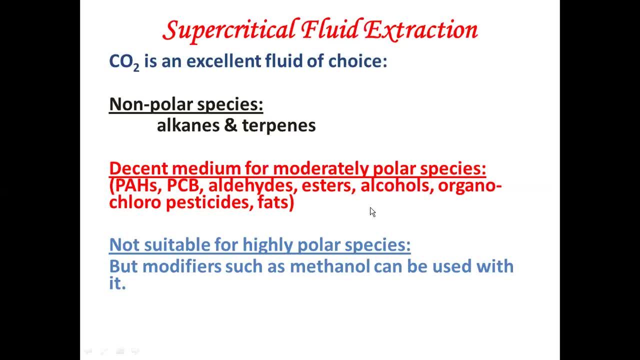 many modifiers can be used along with methanol. when you mix carbon dioxide with the modifiers, this modifiers will modify the polarity of the carbon dioxide. different different modifiers can be mixed with carbon dioxide in order to increase the separation efficiency for different kinds of species. so if some uh the polarity of some. 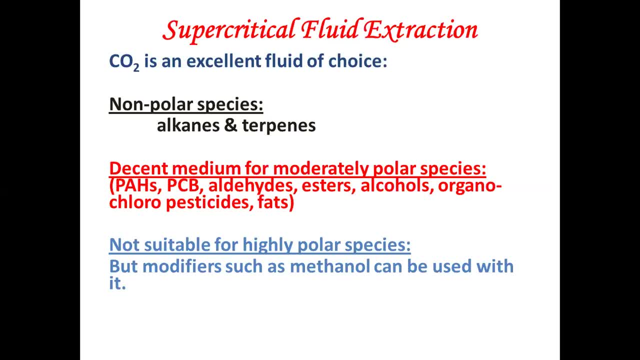 species is lesser than the polarity of the other species. if you mix very little polar modifier with the carbon dioxide and you can eliminate that minimally polar species out from the maximally polar species. therefore, non-polar species can be easily extracted by using carbon dioxide as a supercritical fluid. 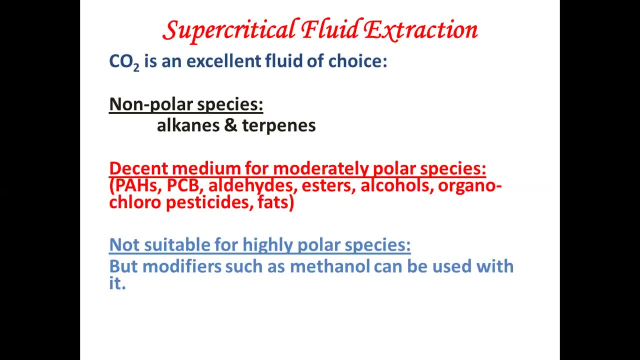 such as alkanes and terpenes, and moderately polar species such as polycyclic aromatic hydrocarbons, polychlorinated biphenyls, aldehydes, esters, alcohols, arganochloropesticides. all these substances, including fats, can be easily separated by means of 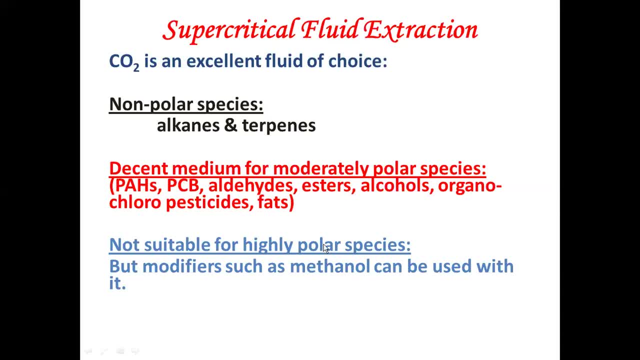 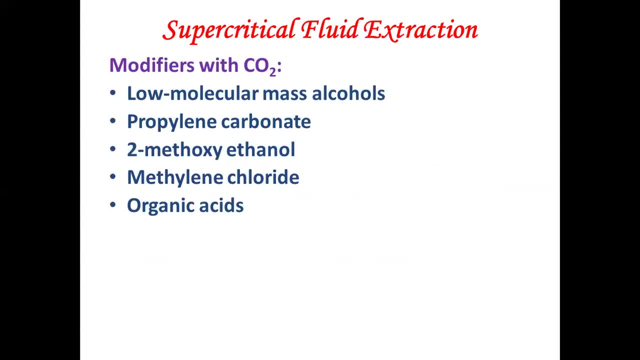 supercritical carbon dioxide, but the polar species can be separated by mixing the carbon dioxide with the organic modifiers. so what are the commonly used modifiers? these modifiers are better to remember their organic compounds if you look at all those organic compounds more commonly. so maybe low molecular mass alcohol such as methanol, or even alcohol. 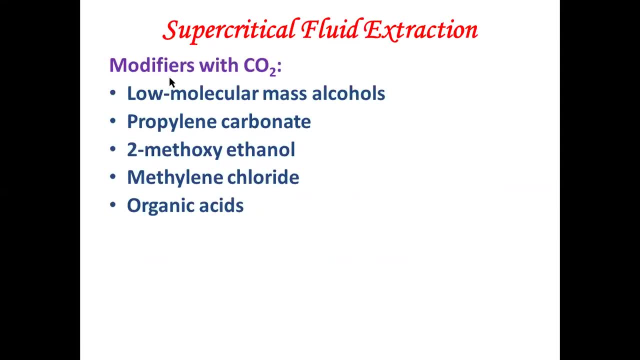 propylene alcohol can also be used. uh propylene carbonate can be used. 2-methoxy ethanol can be used. methylene chloride can be used. organic acids can be used and make sure here they are flammable. the organic, some organic compounds, are flammable while increasing the temperature and 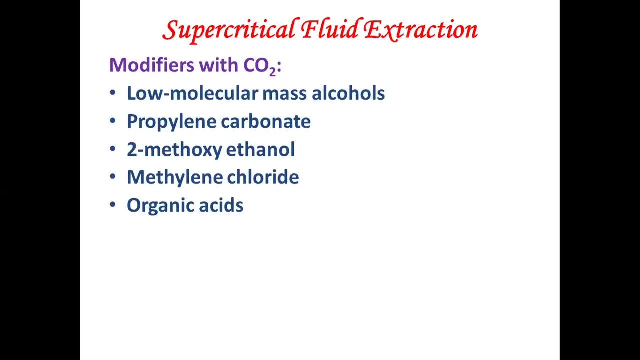 their state of existence must not be disturbed. so modifiers such as low molecular mass alcohols, propylene carbonate, 2 methoxy, ethanol, methylene chloride and organic acids such as acetic acids can also be used, for formic acids can also be used, so when you mix supercritical carbon dioxide. 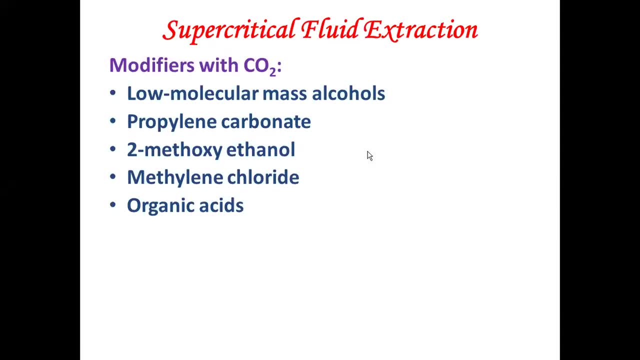 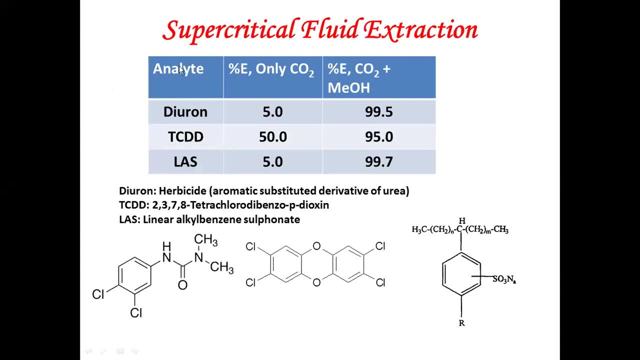 nitrous oxide. with these organic modifiers, their extractability will be increased. if you look at here, supercritical carbon dioxide is used for the extraction of diuron, which is an herbicide and a derivative of urea, and two, three, seven, eight tetrachloro-dibenzo-paradioxin. 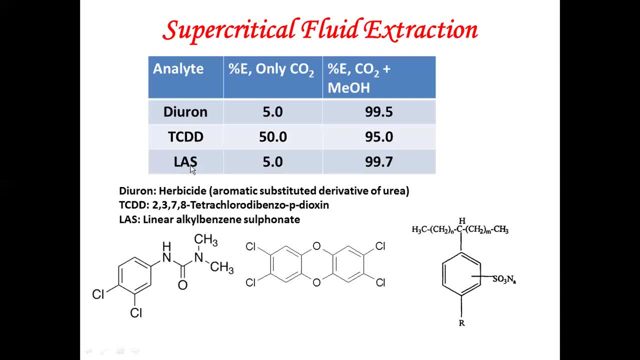 simply tcdd and linear alkyl benzene sulfonate. these are the three compounds which were extracted by using supercritical carbon dioxide and the extraction efficiency values are inside the liquid-bacterium-лекmaster type medium, which is known as the hydrogen sulfide type medium, and the oxygen-bacterium-bacterial type medium is used in alkyl-benzene sulfonate. this is the three components which were extracted uh by using supercritical carbon dioxide and the extraction efficiency values are shown in this paper and the expansion efficiency values are shown here. 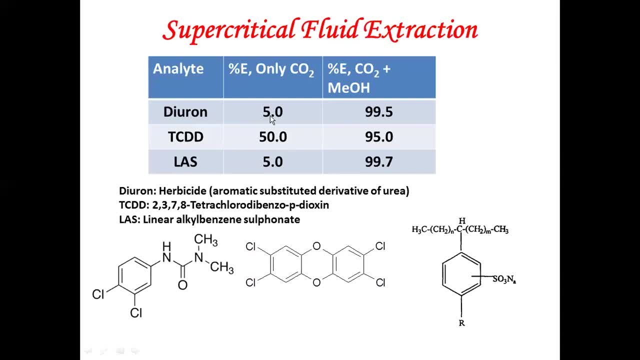 are presented here in this particular table 555, when no organic modifiers are mixed with the carbon dioxide, the extraction efficiency of the urine is 5 percent and two, three, seven, eight tetra chloro dibenzoyl, para dioxin is only 50 percent and the extraction efficiency for linear alkyl benzene sulfonate is 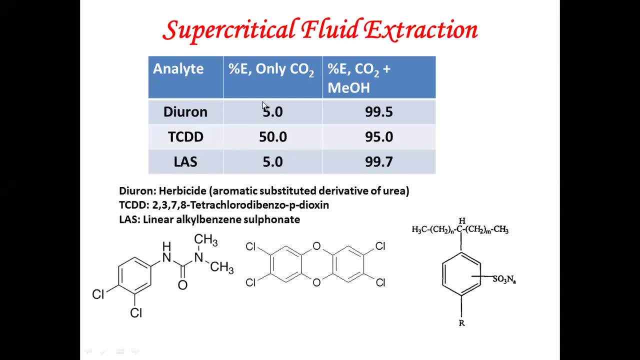 only 5 percent, so the extraction efficiency is not satisfactory. how to increase this? because of non suitability of carbon dioxide and it's non polarity, the extraction efficiency might be lower. so what we can do? the polarity can be modified by mixing with organic modifiers such as methanol. supercritical. 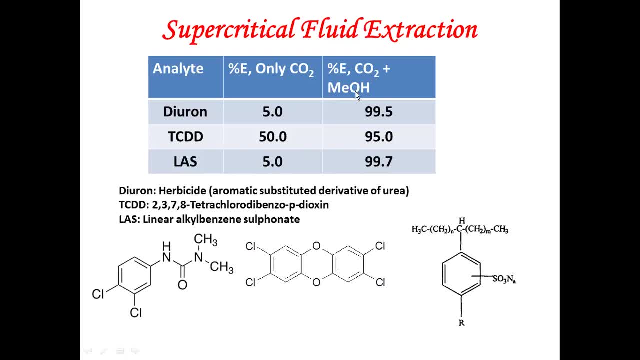 fluid, carbon dioxide is mixed with methanol, again supercritical fluid state is attained. if you look at the extraction efficiency, the urine is extracted up to ninety nine point five percent. TCDD is up to ninety five percent extracted linear alkyl benzene sulfonate, extracted up to ninety nine point seven percent. so in the